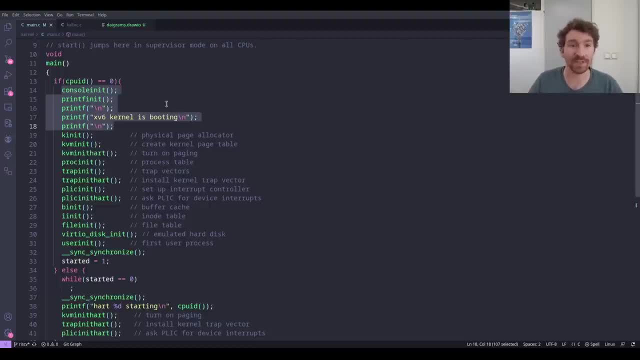 kind of ready for the operating system. then we're into the operating system and we prefer get everything we need to actually print stuff to the screen up and running as soon as possible so that we can actually kind of debug the system and get some some useful information. 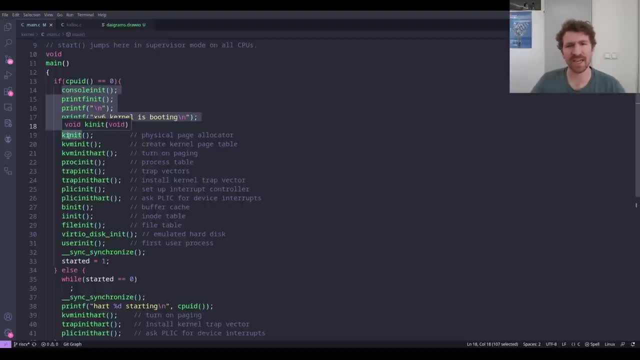 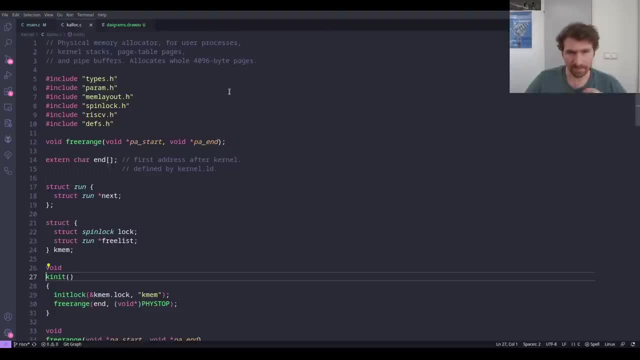 out of it. That brings us to this KInit function, which is labeled as the physical page allocator. So let's take a little um, a little walk into this. So this is actually quite a small file. there's there's 83 lines of code in this file, um, and the comment up top says: physical memory allocator for user processes. 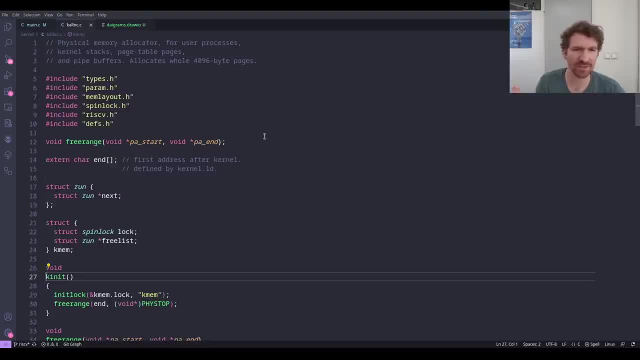 kernel stacks page tables- page table pages rather- and pipe buffers- allocates whole 4096 byte pages. so that's that. that's what it does. we don't have to understand what all of that means right now, although hopefully by the end of the video we'll be able to understand what all of that means. 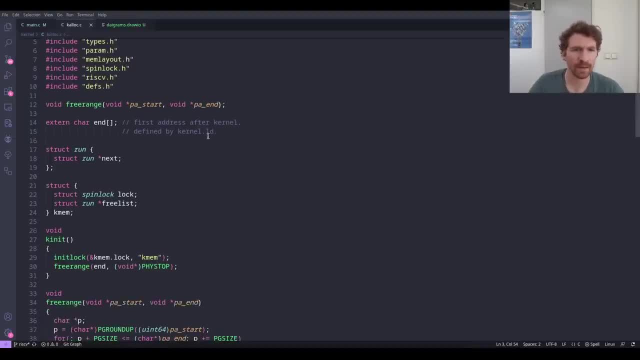 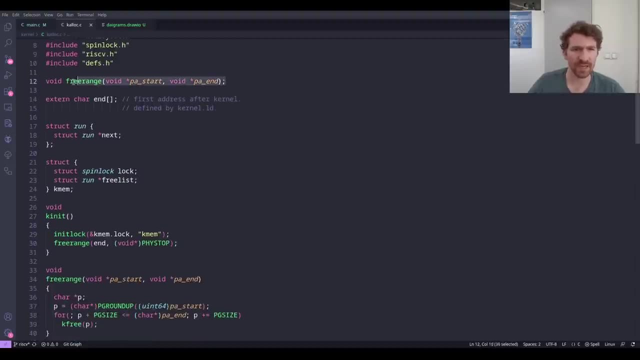 This will understand at least the most important parts of it. okay, so we bring in some, uh, some header files that are stacked around. we'll go into some of these. uh, we declare some functions up top so that when they actually get called before they're defined, that's possible. that's just something you 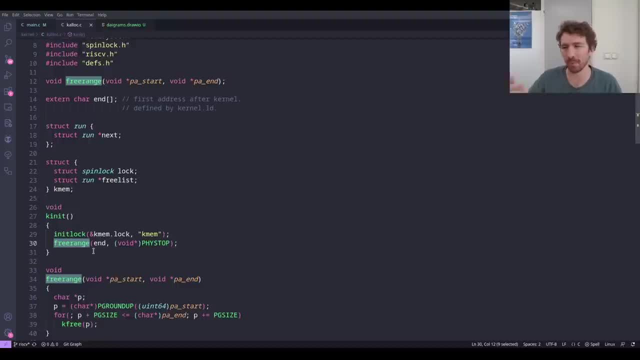 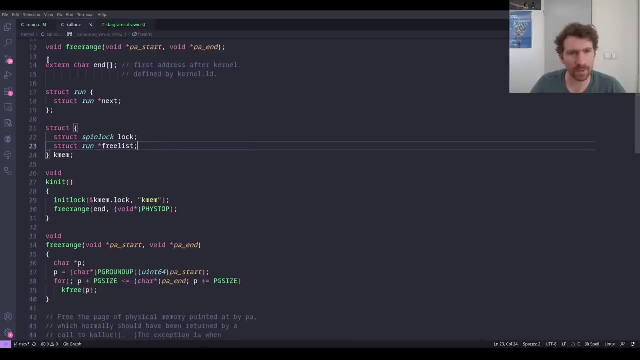 need to do and see, like, if you use a symbol before it has actually been like kind of defined within the um, within the file, you kind of need to kind of declare it up top somewhere, A forward declaration of that um. next we have, uh, an extern car end array which is actually 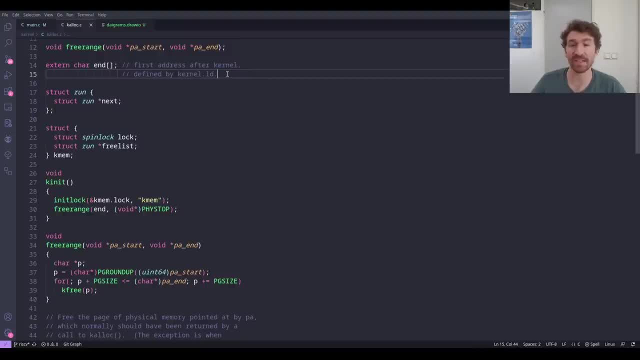 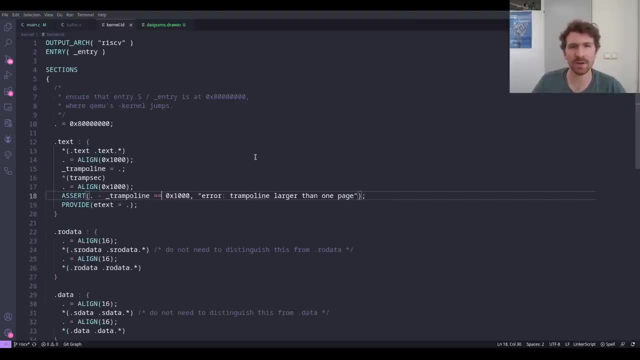 labeled here as the first address after the kernel defined in kernelld. we looked at kernelld in the in one of the first episodes, but, um, it's a good time to come back and look at it now. this is the linker script, so this is what actually tells um at the final step of 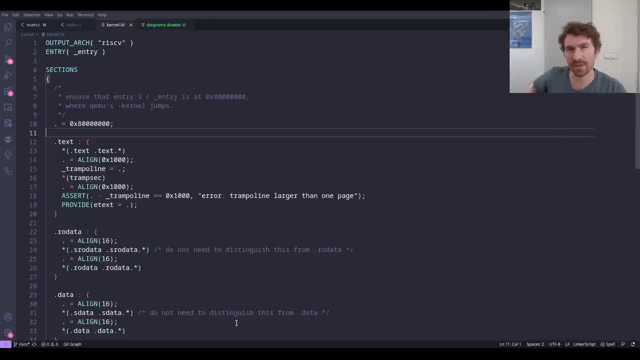 when we've compiled all the individual translation units, all the individual c files and assembly files in the system, we have to link them all together. this is the final step, and this linker script is kind of provides a guide of how we, how we do that. it's a kind of a set of restrictions. 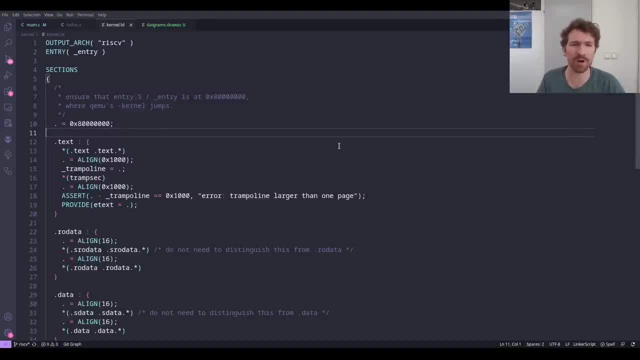 that we have to have to have from our final output program and like, for instance, that everything will begin, uh, kind of reference to this address, which is the beginning of ram, because of course we're going to load this program into ram. so if we talk about there being a certain like, we're jumping to. 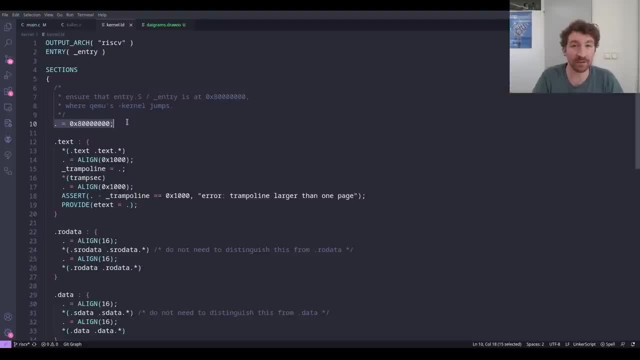 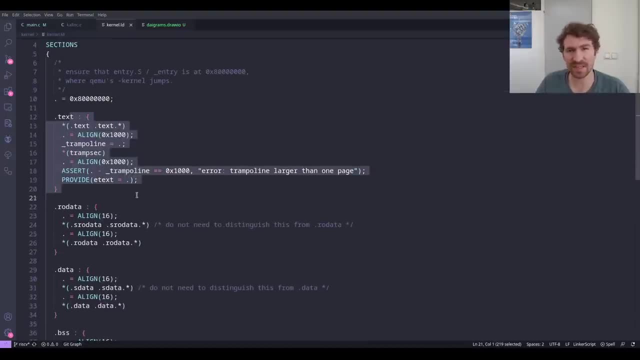 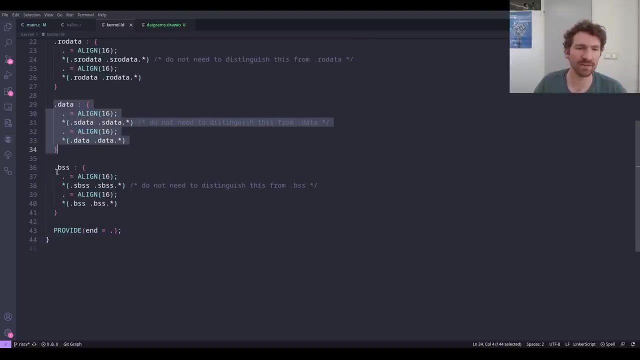 a certain address. it's all going to be sort of calculated relative to this very first address. then we have the various sections. so this is the text section, it's code. we have the read-only data, then we have the data that has been initialized, then we have the data that has not been. 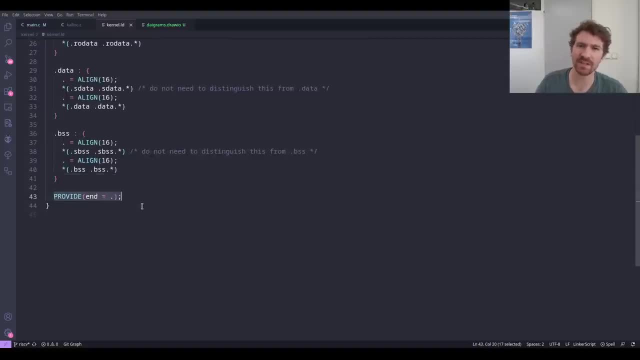 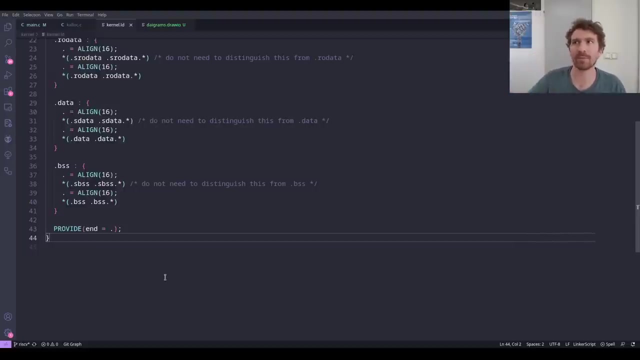 initialized and then what you can see is that there is this statement at the end that says: provide end dot equals dot and, in kind of linker script, uh lingo. what this actually means is: the dot is always tracking where you are right now, within sort of like providing relative addresses. 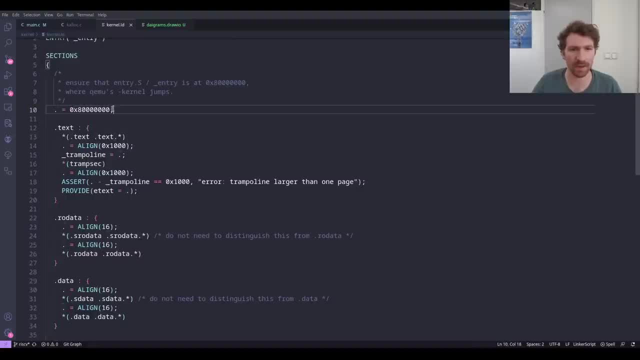 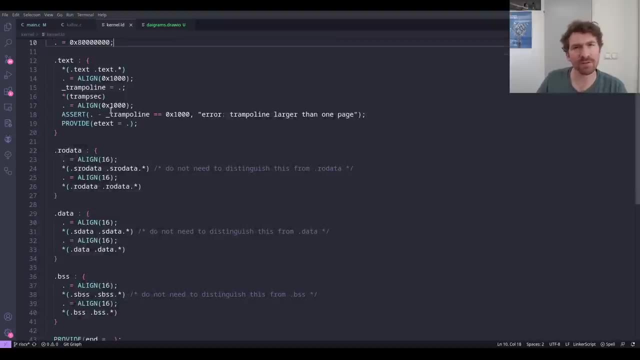 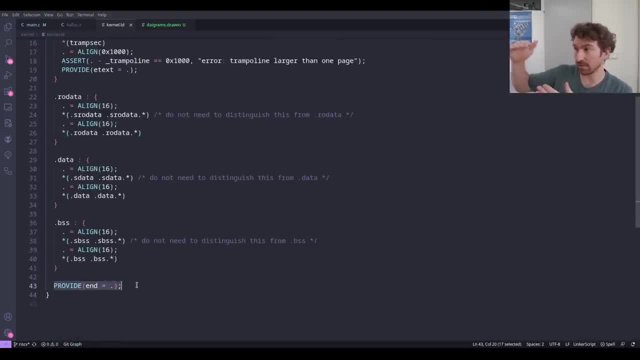 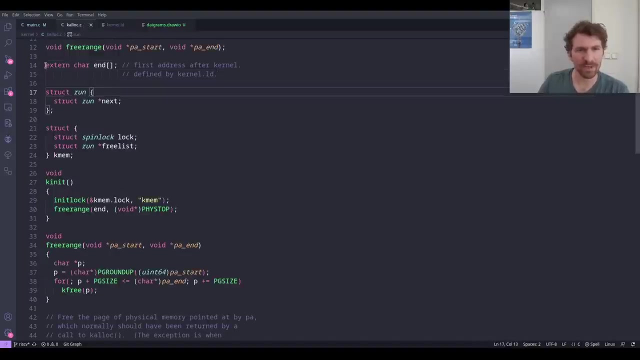 so by the time we get down to this point, that address is kind of it has been incremented a whole bunch. wherever that lands, wherever that happens to be at the very end of this, we mark it as the end and we provide that as a symbol. so this end. coming back to k alloc, when we see here this: 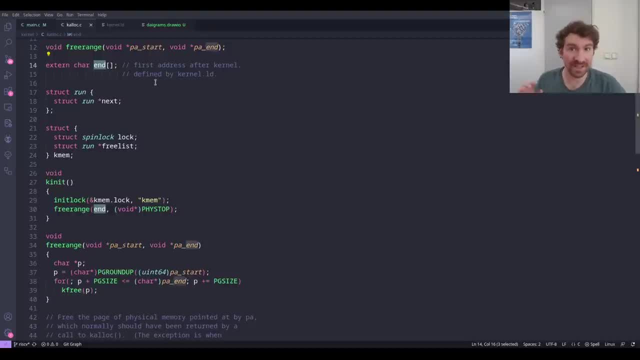 extern car end. this is actually referring to this symbol given by the linker script. so it's not a symbol that actually exists in the code. it's a symbol that's kind of injected during the process of linking um and kind of the way it's set out here, declared as an array, is just a convenience. 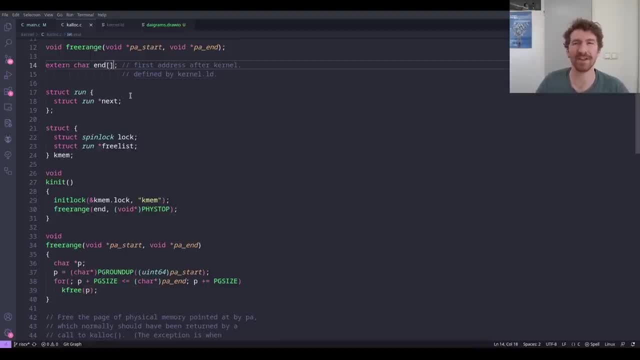 to make sure that when we actually access it it behaves like an address. that's this the short way of putting it. if you experiment around with linker scripts and kind of providing symbols, you'll see that the symbol is provided um, but you have to kind of take its address to get the value. 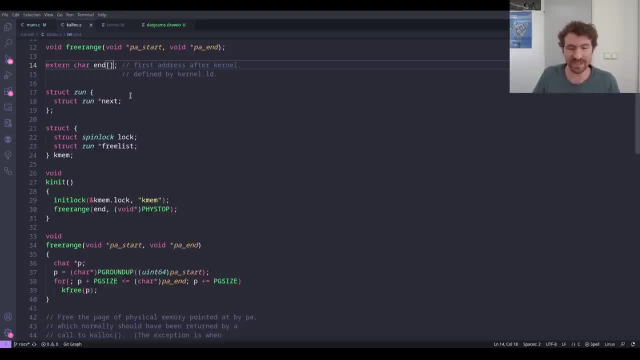 you're after, like what we want to know is: where is this, what is the end, what is the last address of um? and by kind of uh, putting these array brackets, so kind of saying that this thing is an array, this is a very simple way for us to to do that. okay, so this is just just getting that out of. 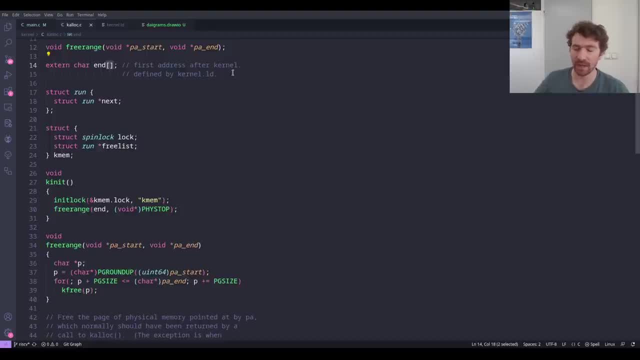 the way we now know where the very end of the kernel is and keep, keep in mind- here that's tracking all the code of the kernel, but also, after compilation, where all of the variables are going to go, where all of the read-only data is going to land, and 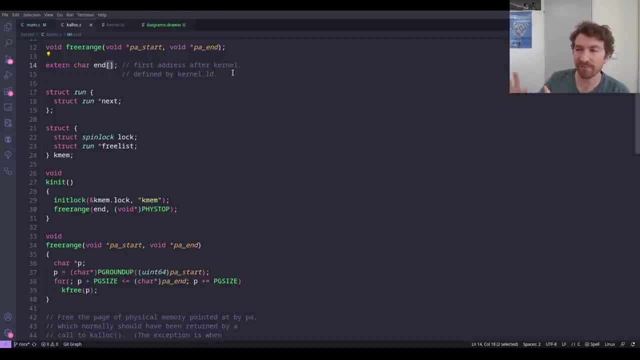 like where any, just anything else like that. so basically everything as we know it when we compile, the program gets us to a certain point. everything after that is kind of free memory. right, it's everything from the end of that kernel until the end of physical ram. that's what we've got. 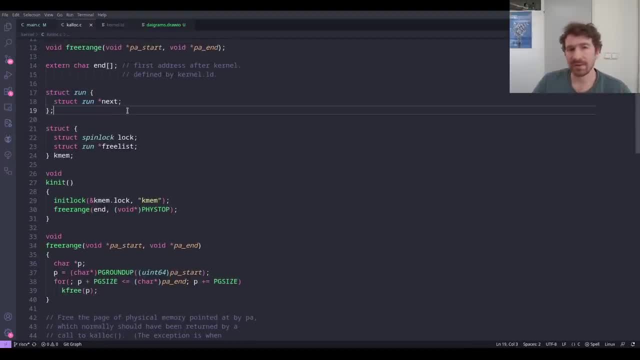 to play with at that point. next, there is a definition of a structure. it's called run and it's a weird little structure. um, it's a structure that basically contains one memory, so it's got like kind of, if you're coming from a high level language, it's kind of like an object. 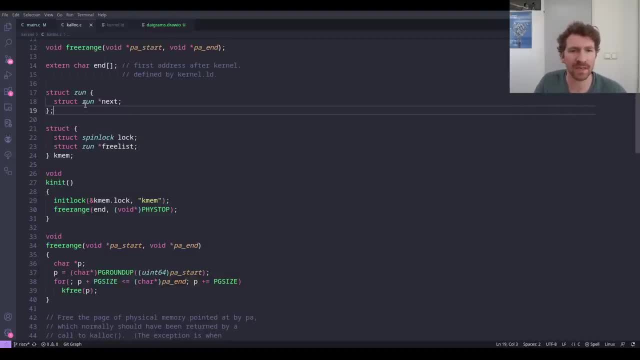 with one member inside and that member is a pointer to another structure of the same type. so, uh, and you'll notice, it's called next. this is basically the the most minimal linked list implementation you can imagine. it's like a linked list that doesn't even contain data, it's just. 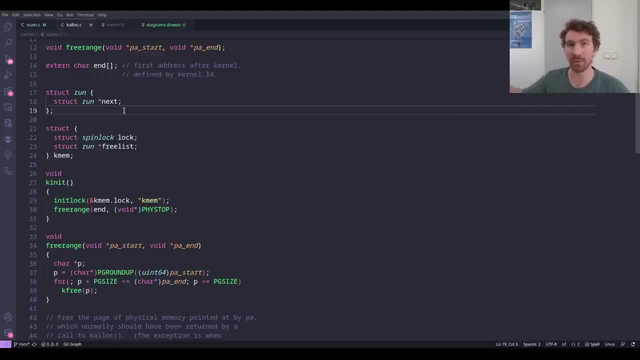 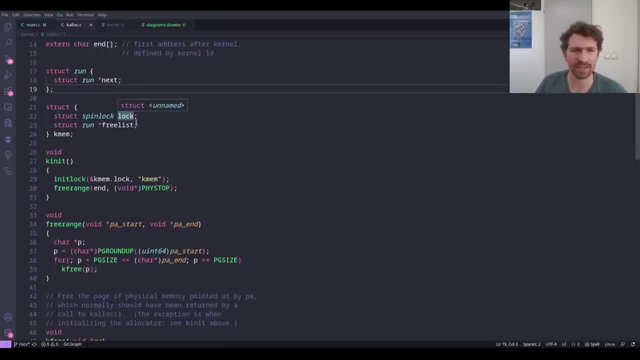 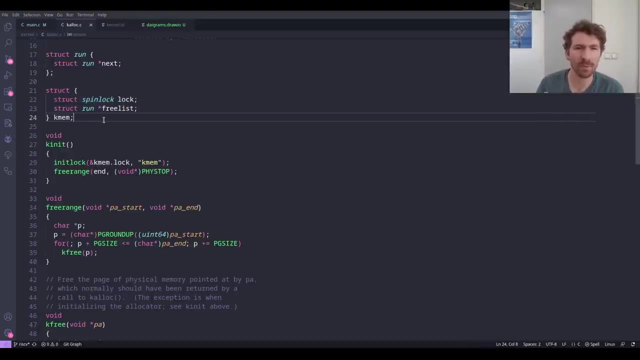 purely one thing pointing to another thing pointing to another thing. it's kind of a bit of a weird, weird concept. you have to wrap your mind around it a little bit. we'll see how it, how it gets used. next, of course, we've, uh, we've got kind of like a little um, a little piece of data. that wraps up all. 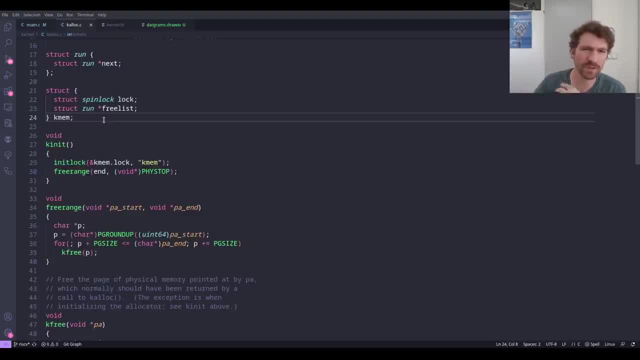 of the interesting things that we have in this module. so it's called km and it keeps track of the spin lock. of course, we've seen spin locks. now they are used throughout the operating system to make sure that we have mutual exclusion on resources. basically, we can use this to make sure that any multiple cpus in the system which 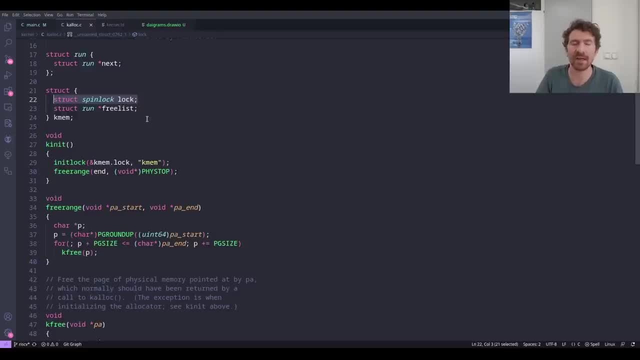 are going to try and access, say, the page allocator, they're going to have to take it in turns. right, they're not going to be able to come and all try and do the same thing at the same time. they're going to be forced to take turns, uh, to do this. that's what spin locks are all about. there's a 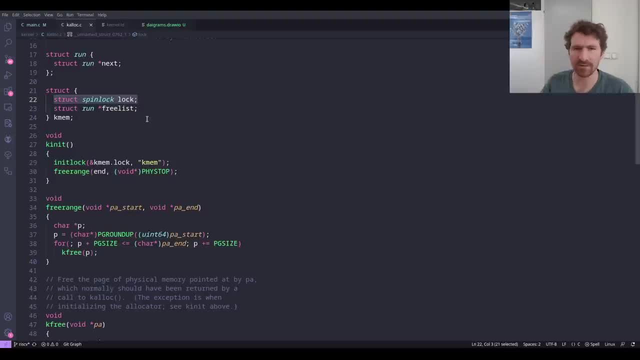 whole episode on spin locks if you want to get a bit more into it, but for now we can just use them as a tool. right there are. they're all a tool for mutual exclusion. so if you want to get a bit more into it, but for now we can just use them as a tool, right there are. there are a tool for mutual 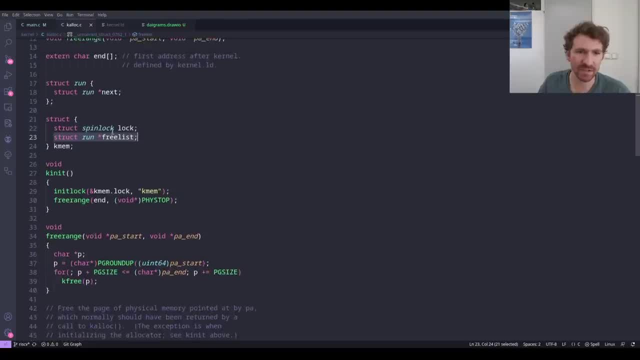 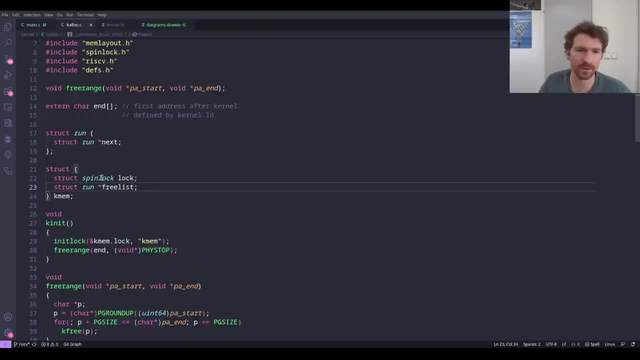 exclusion, and next we have a pointer to a one of these structures called the free list. so it's we now here. what we have is space for a pointer, so not actually a structure in this thing- a pointer to one of these structures and, uh, that structure of course. then if we kind of read through whatever 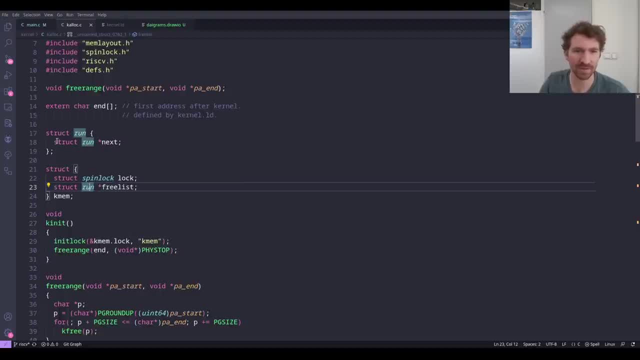 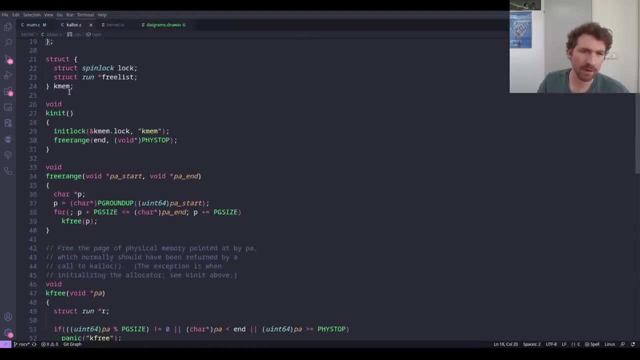 we had. if there was a value in here, we would have some access to some next piece of memory, that's, or next structure, rather we'll. this will become clearer. if this isn't clear to you right now, that's fine. like this, this will become clear, all right. and then, finally, here we have the k. 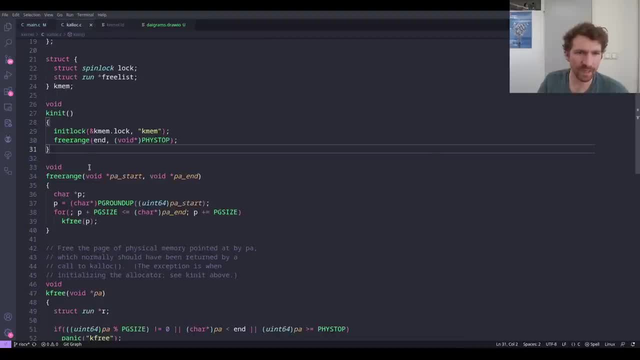 init function. so this is what we're actually running here, uh, so k in it. what do we do? we, uh, we initialize the lock standard stuff. we've seen that. then we call this function free range and we, if we look down here below right, free range is a. 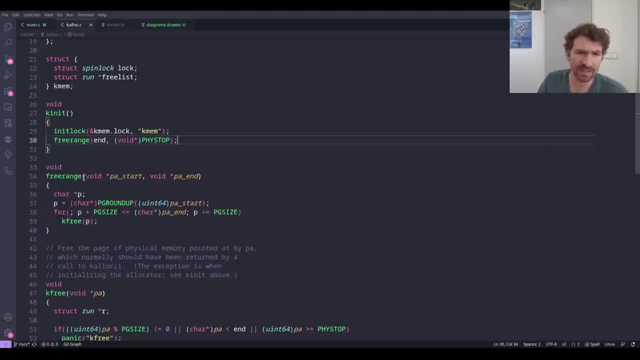 function that doesn't return any items, it's void, and it takes in two parameters. it takes in a pointer to pa start, that's a physical address start, that's the start, the physical start address that we want to free. and then there is a pointer to a pa end- a physical 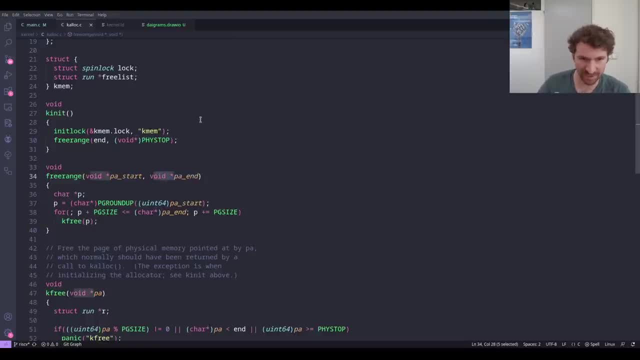 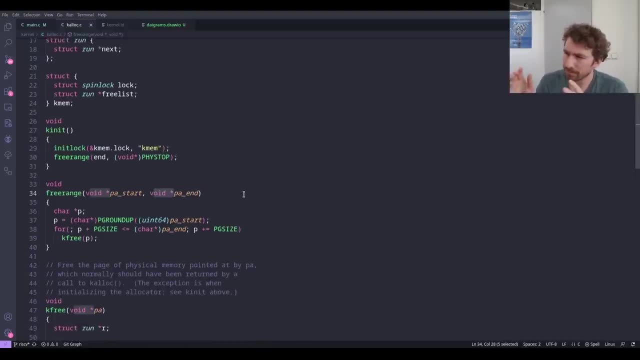 address end. now notice what we pass in here. these are both void pointers, right, and a void pointer is just. it doesn't actually point to any particular kind of data, it is just a sort of free floating address and this is c's kind of um most low level generic type. there is actually the void. 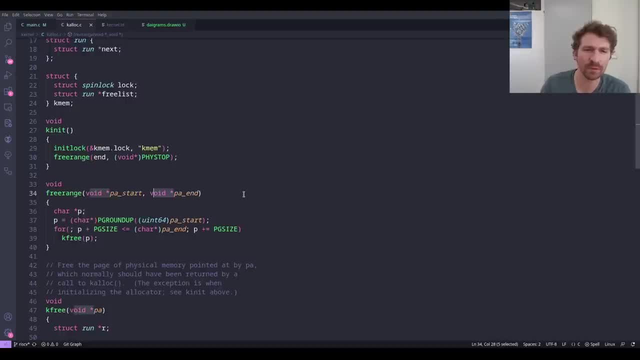 pointer. um, it's basically a way of like, but if you want to use a void pointer, you always have to cast it to something, so you have to. you actually actually have to say what the data is this thing points to. but, um, this is often used in the case that like. 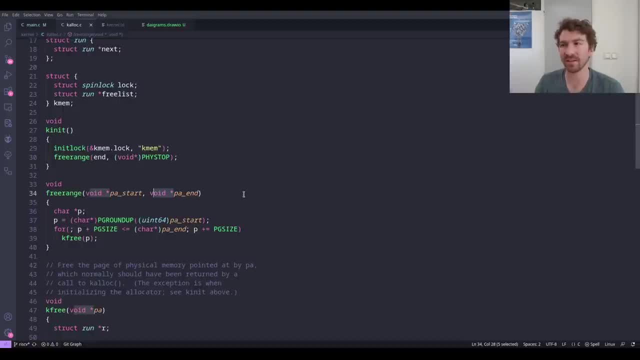 you're referring to is is actually not as important as the fact that you have just an address to something. so that's why we're using a void pointer here, and you can see that what gets passed in here is the end. so that's where we start, the end of the kernel, like 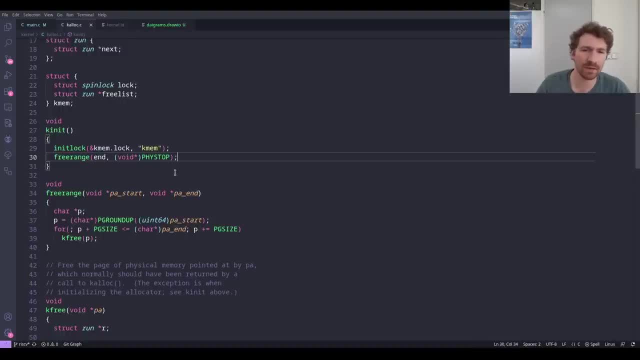 after all of the kernel stuff, and where we uh, where we end here. the pa end is confusing because pa start is end here, but pa end is uh. is this define here phi stop, which is presumably phi physical stop, the physical end of memory? so let's go to that define here. that brings us into mem. 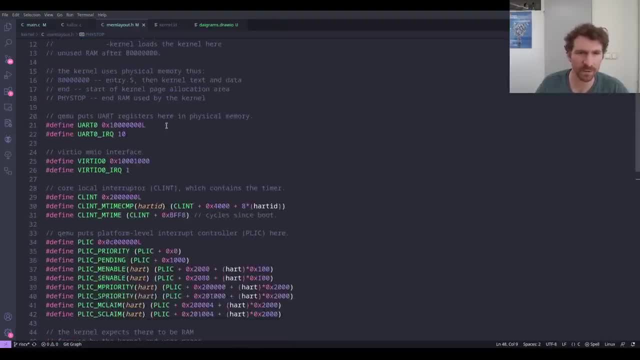 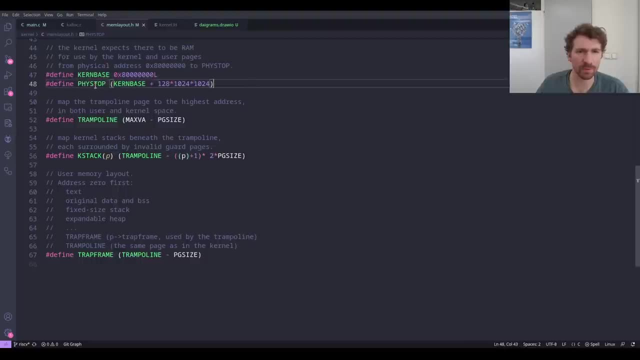 layout, dot h, which we've actually seen before a couple of times now. um, so down here we have the this, this whole calculation for where the, the physical, the physical top- sorry, i'm saying physical phys, physical stop, and i think it's physical top, like the top of physical memory. this is why 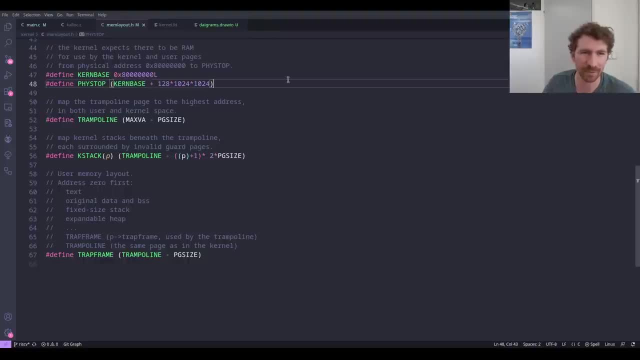 naming is actually important. uh, and try try to not be so ambiguous, but basically what this define is giving us is, like the, the sort of the very end of ram, like okay, we've got this much ram, that's it. 128 megabytes in the default case of xv6: 128 megabytes, that's the end of ram. so the way this is computed is we? 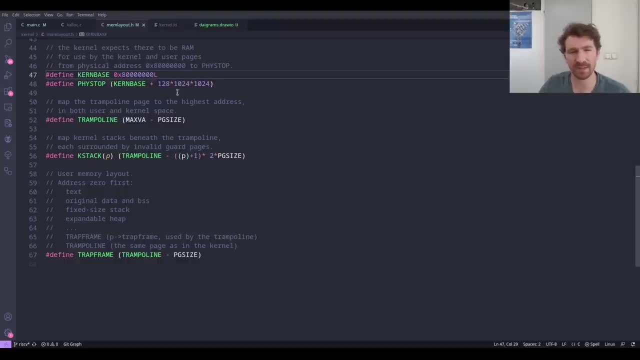 know where the kernel starts. that's this address: 80 million. that's already been kind of um kind of explained. so the end is well, that kernel base plus 128, multiplied by 1024, that's going to give us 128 kilobytes. and then once again multiply that by one- 1024, that's going to give us one that. 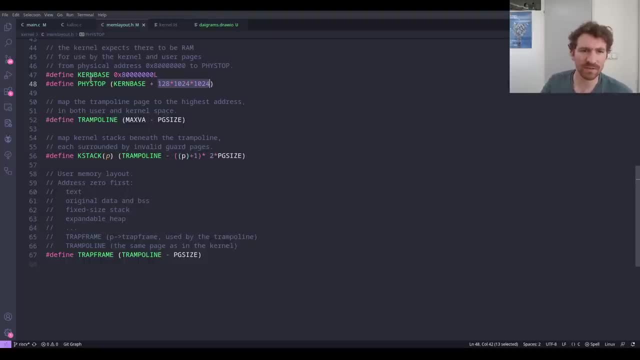 128 megabytes. so the physical top of memory of ram is the, the kernel's beginning, plus 128 megabytes. that that should make some sense. it's basically just it's. it starts here and then we have 128 megabytes of memory. so wherever that ends up, that's the end of memory. so what this statement? 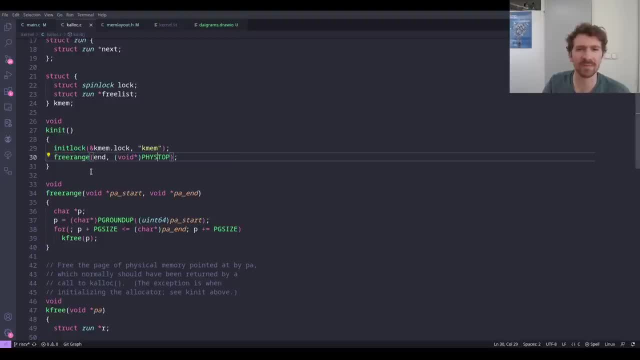 is telling us is that we're going to try to free a range of memory that starts here, at the end of, kind of wherever the kernel finishes up, that point, uh, all the way to the end of memory. uh, so what are we doing here? we're going to be preparing all the free memory that we have, that's. 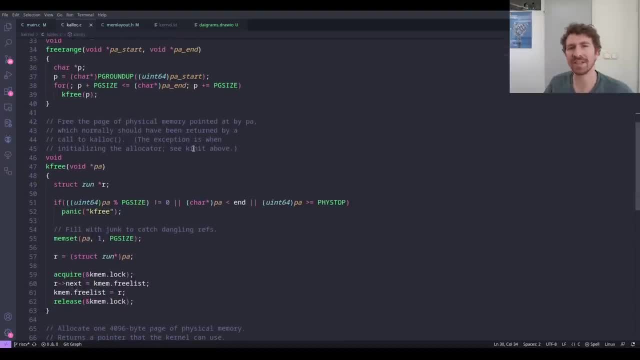 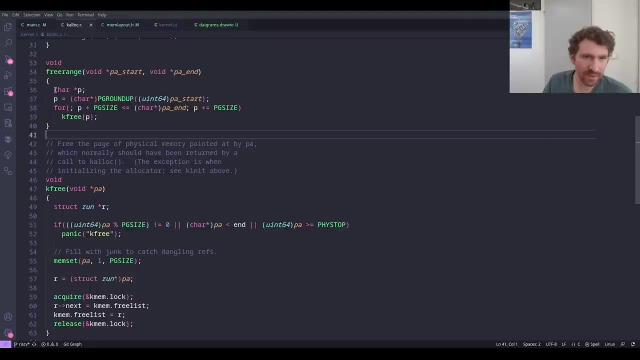 what we're doing. that's the idea. so, free range. what does this function do? um, what this function does is it calls: um, well, we start out with a character pointer, so that's just something that's pointing somewhere. uh, it's just kind of a free variable that gets used, uh, in the loop, so that 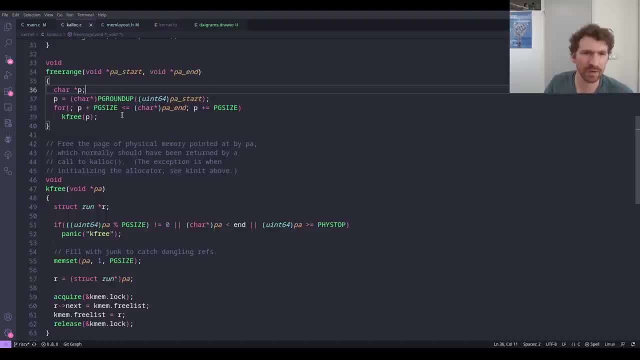 we don't have to do anything weird with with other variables. so we've got this character pointer and we assign it to uh the physical address. start, um, cast to a uint64. so this is a void pointer. now we're casting it to a uint64. that makes that takes, gives us the address as just a regular uh integer, basically. and then 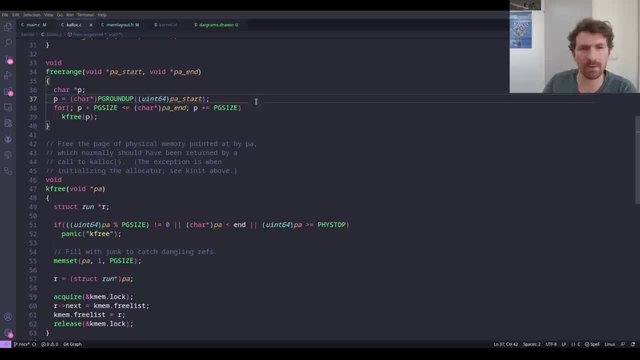 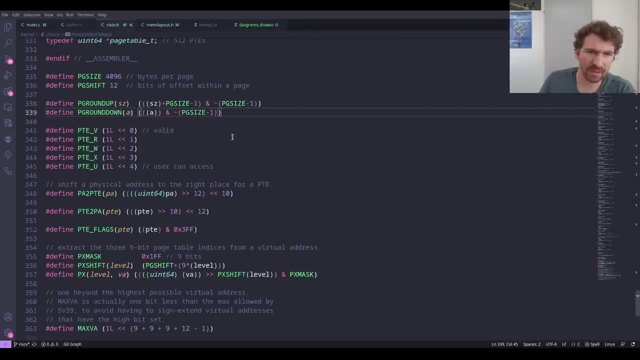 we're using this macro- pg roundup, um- so let's go to that because that's going to be important for us to understand. so, pg roundup size. it's a complicated looking piece of code and i've actually explained a piece of code like this. uh, exactly, i walked through the whole macro in the bare metal programming series that i've done. 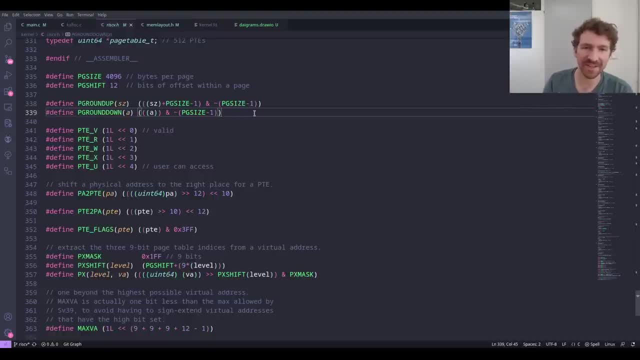 i'm not expecting that you go off and watch that whole series to understand this, but basically what this does is this rounds up to a certain size. so let's imagine to this, like we passed in um, this comes to this어 and this Pg roundup for the %: PEG round up question. 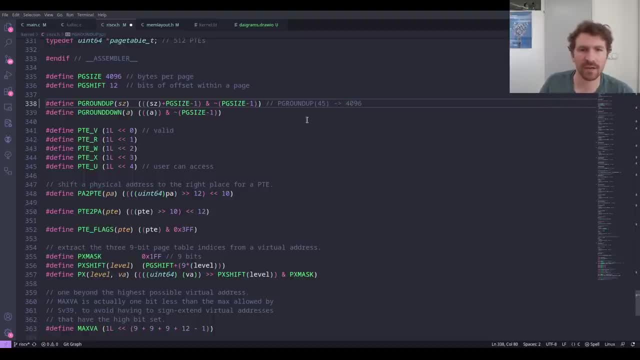 g75, let's say we- that's the number we passed into this- DIE SIMİ T k. the outcome of this is going to be four thousand ninety-six, because we're rounding up to the page size. that's the idea here. if we're, if we're not on a boundary of the page size, so if we're not 4096, or two times 4096, or three times 4096 or some multiple of 4096, 4k. 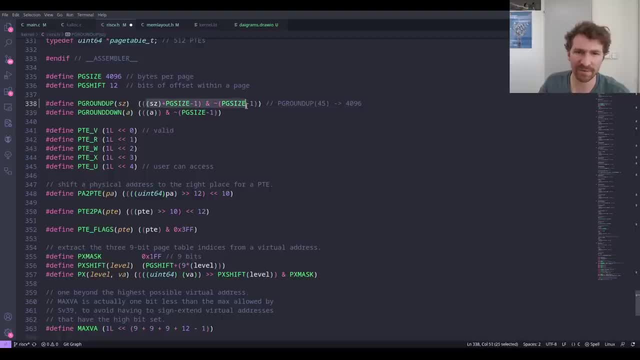 If we're not on a 4k boundary, it's going to round up to 54len IV3 Online 2020, which is up, And using this little bit of bit math that's defined here, it does that If you kind of want. 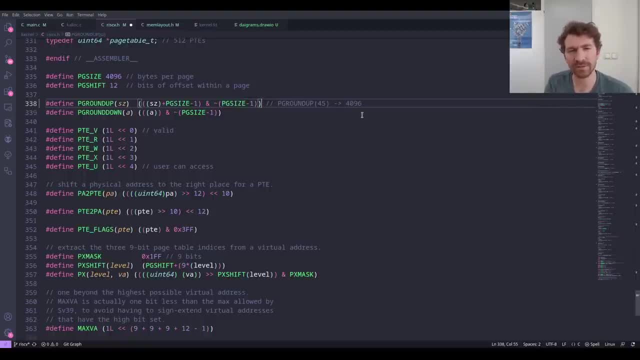 to figure that out. I'm not going to explain it now because it's just going to take too much time, but copy it out, put it into a C file or whatever programming language you want to experiment with and play around with it. And the mechanism, if you sit down and you work out what's going on. 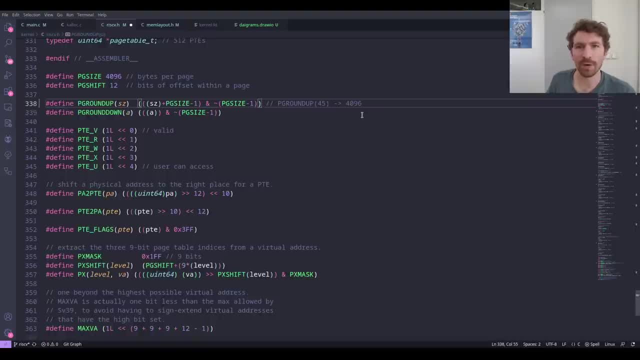 at the bit level by converting all your numbers into ones and zeros. you'll see that this is actually a really elegant way to round something up to a particular boundary, And it will only work in certain conditions, so you'll also be able to see that as well. But in this case we're going. 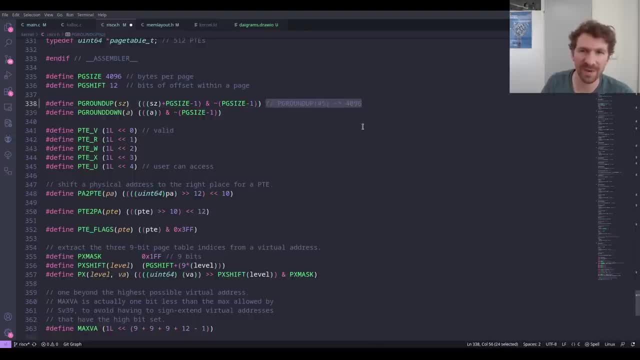 to be going up to a 4k boundary. That's the point of that. So what's this whole thing about 4k? Because we've seen it a whole bunch of times now. right, We've seen the idea of this 4k in the stack and in other places, Well, in operating systems. 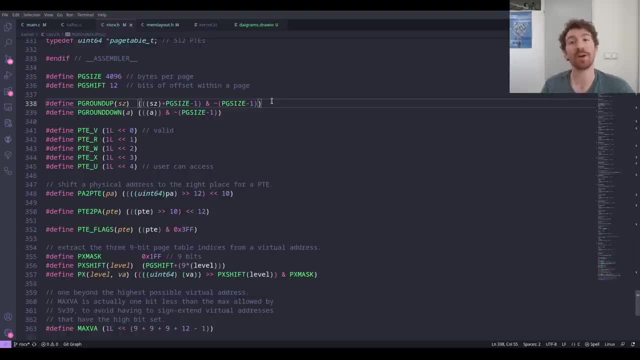 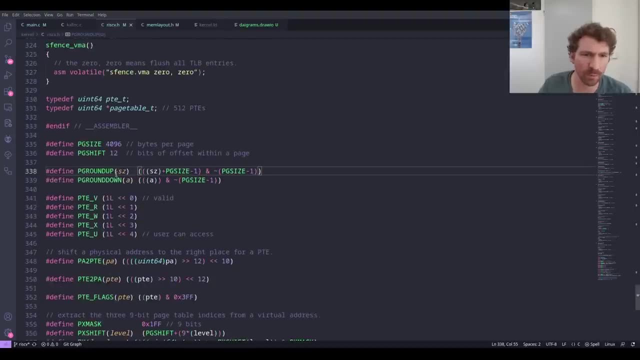 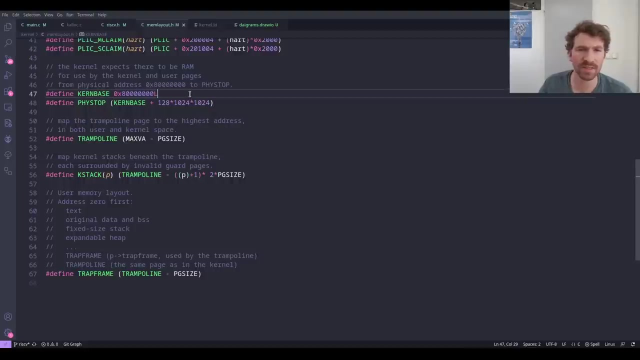 you have something called virtual memory. Now, virtual memory is the idea that you have physical memory. right, We know that, for example, the assembler- sorry, the assembler- the kernel starts at this address. This is a physical address, right, This is an address on the machine that. 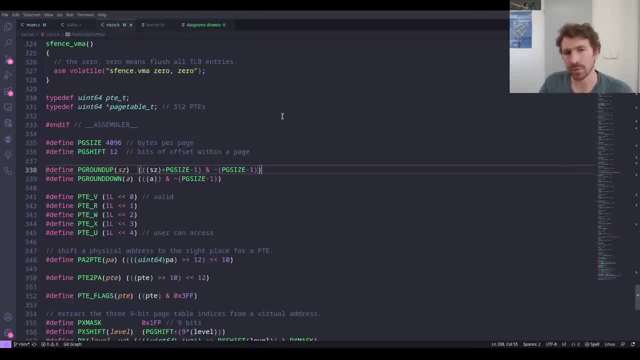 it refers to something. A virtual address is something where you first have to go through a translation step in order to get to the virtual address, And you have to go through a translation step in order to get to the virtual address- physical address- And the benefit of this, or the point of it, in fact, is that we can use 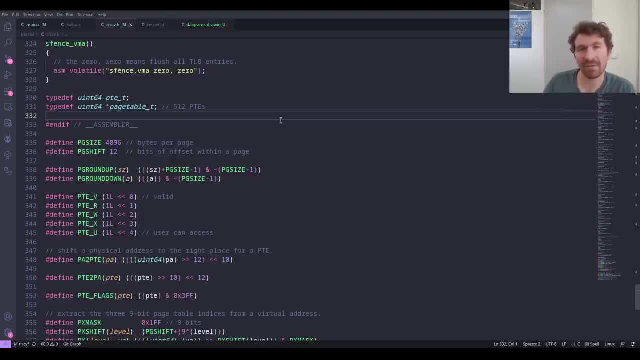 this virtual memory system to have process isolation in user space programs, or it's one aspect of that at least. So the idea is that any given user process to the user process it appears that it has its own full computer. It is the only thing running. It has access to an entire memory. 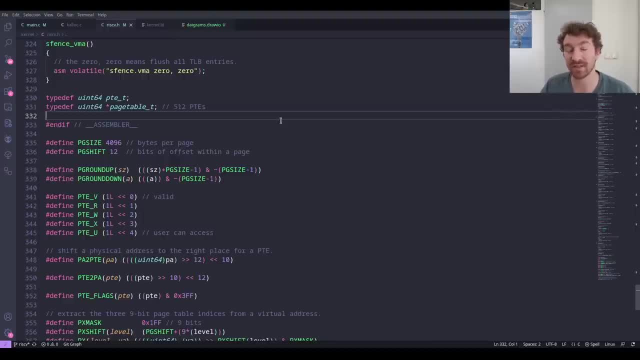 space And it has access to a whole bunch of other things. So it's a virtual memory system, But all of its memory addresses are translated to physical addresses through a process called virtual memory address translation, And that happens with a whole mechanism that involves. 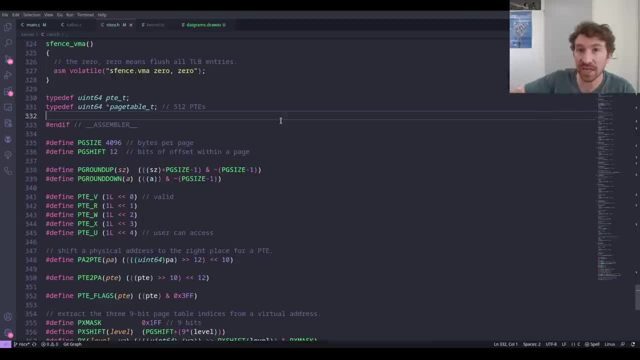 stuff on the CPU. It involves page tables in memory. But the point I want to get to here is that pages are kind of the unit of virtual memory. So if I have a virtual memory address, the way that it kind of ends up working is through that. 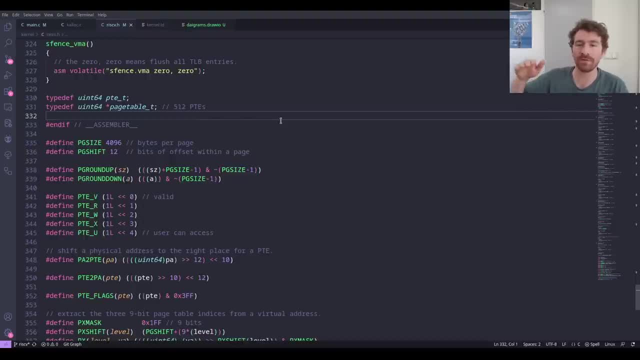 translation process, it always translates to one 4k block. Now, not to make things too confusing, but it doesn't have to be 4k, right? That's a sort of machine specific thing, And it just so happens that on many, many systems, including this RISC-V system, including many x86 systems, 4k is the 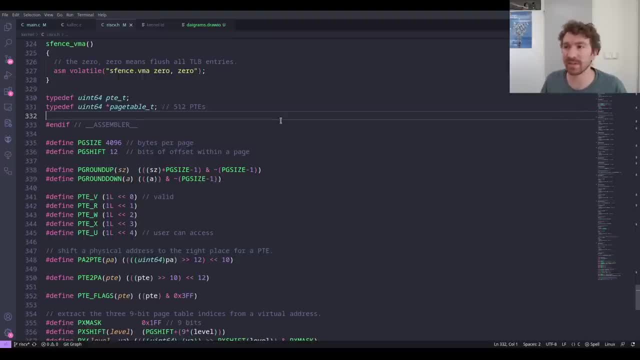 standard page size. But on other systems like the Apple, the new Apple Silicon, they actually have a 16k page size. So it's they have big, bigger pages there. But the idea is that when you're doing virtual memory you it's done in blocks. those blocks are 4k each And an address. 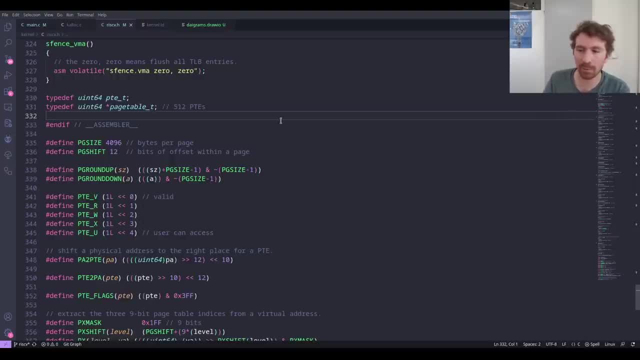 trans and any address that you try to translate is always basically going to point to one of those blocks plus some offset within that block. So you can't like, you can't give a process or anything. you can't actually give a process: more sorry, less memory. 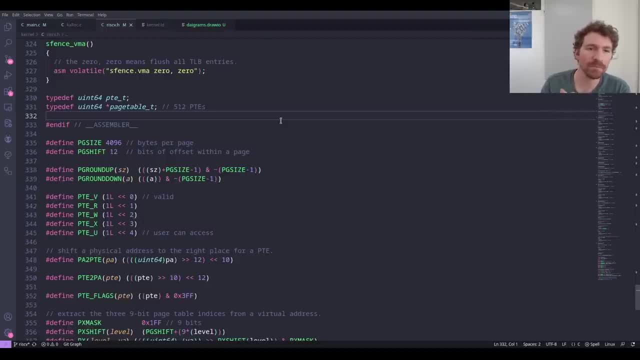 than 4k. Like that's the minimum. Of course you can always build other mechanisms around that, But like that that's the point right. When in the system doing address, translation, multiple processes, 4k is the sort of the minimum unit. So the kernel also works in the kernel also works. 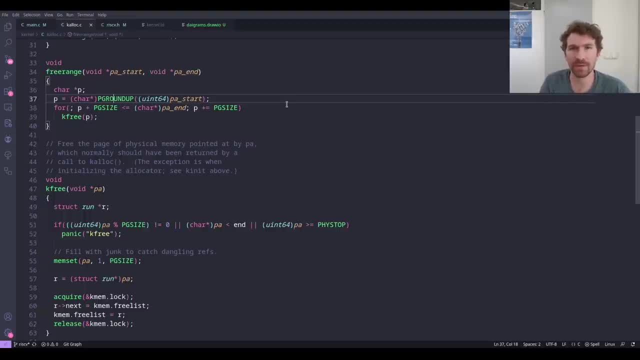 in units of 4k, because that just makes everything easier with address translation. right, If you make sure that everything that you're allocating lines up on a 4k boundary, you can just perform this address translation way easier. I'm not even sure if it's possible. 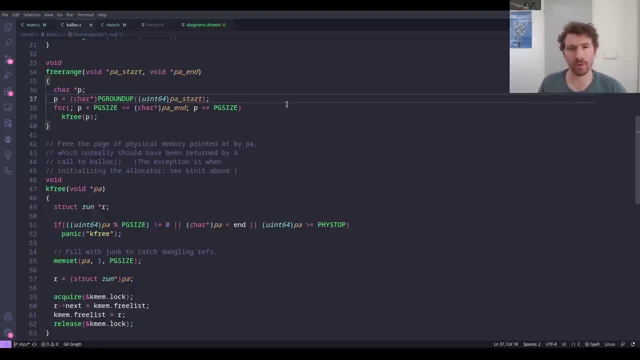 to do it without kind of making sure everything lines up on the form of 4k boundary? probably not. I haven't really gone through the process of thinking that through. So in the end what we have now is the start address rounded up to the nearest 4k block right. 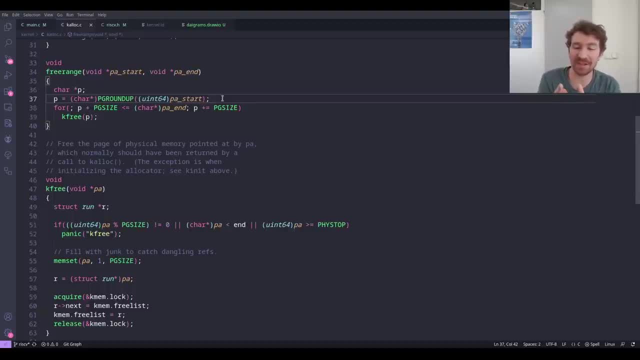 So all the memory that happens before that, there's going to be this little block of memory between the like, the end of the kernel and the rounded up thing. that's just sort of dead memory to us. we're not going to use. that doesn't get used for anything. That memory is lost to us. 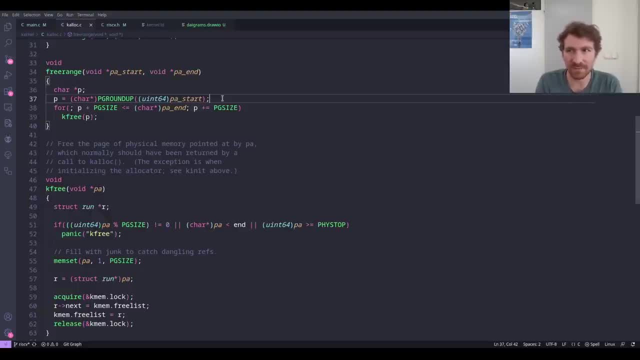 but it's going to be a maximum of 4095 bytes, right? So it's not that much in the grand scheme of things. in terms of 128 megabytes, I mean, it's not insignificant, but it likely won't be the worst case. And then what we do is we iterate using a for loop. So 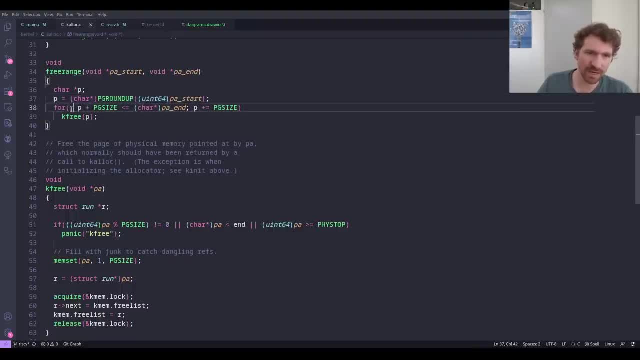 for we've already initialized our value, So we don't do it there, But we could have moved this p here, While p plus the page size, which is 4k, is less than the physical end address that we are dealing with. 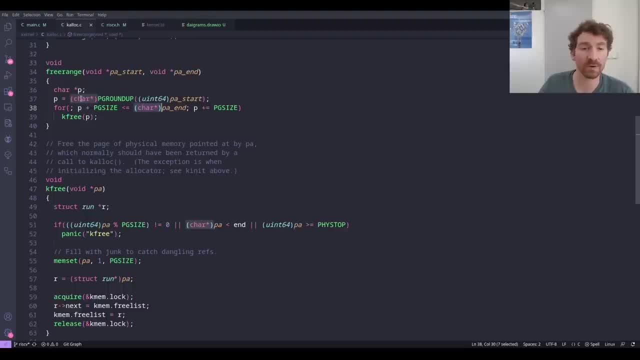 Cast to a character pointer, because then we can actually compare them in an accurate way. P plus equals the page size. So what we're doing is we're looping through and every step of the loop we are incrementing our pointer by 4k, So we're jumping to the sort of the next page. 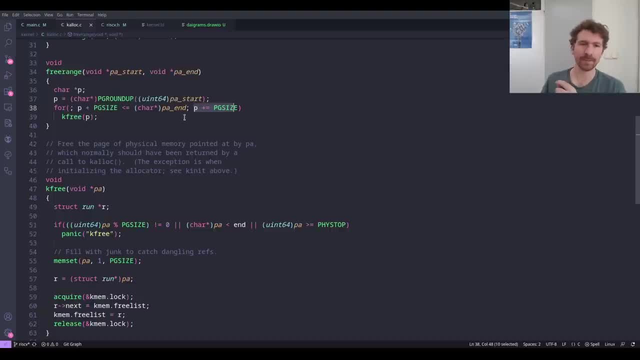 And we end up calling this function, called k, free. So this is a page allocator, right, And what we're actually doing now is setting up all of our free pages, like when the system boots. all of the pages in the system should be free. we haven't. 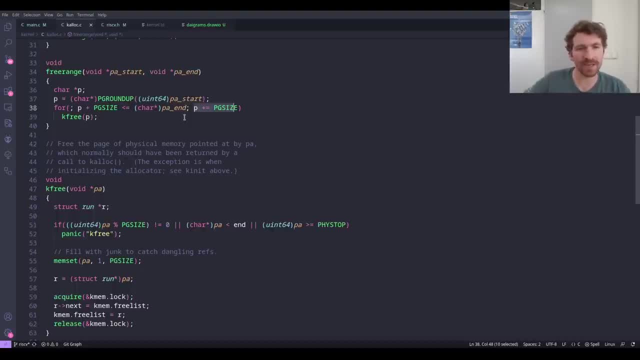 allocated any memory yet- But the process of getting to like a big list of free pages. we actually do that by piggybacking on our page freeing process, So it's quite clever in a way. we end up calling the same k free. 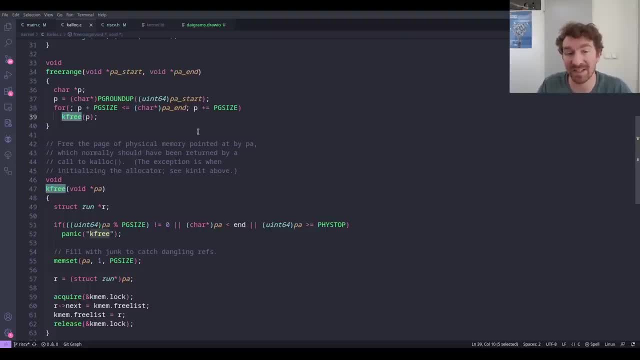 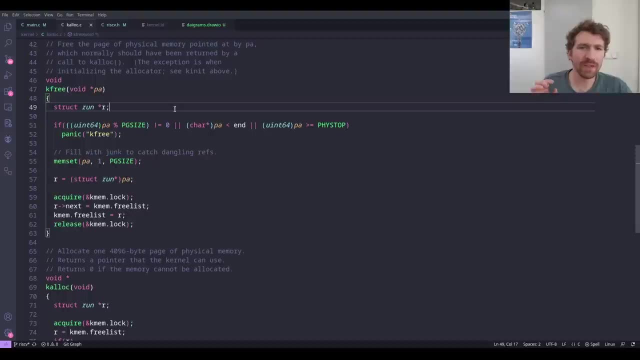 So we call k free on this pointer. that brings us down to this function: Free the page of physical memory pointed out by the PA, the physical address, which normally should have been returned by a call to k alloc right. So like getting and freeing memory is a two step process. First you get memory. 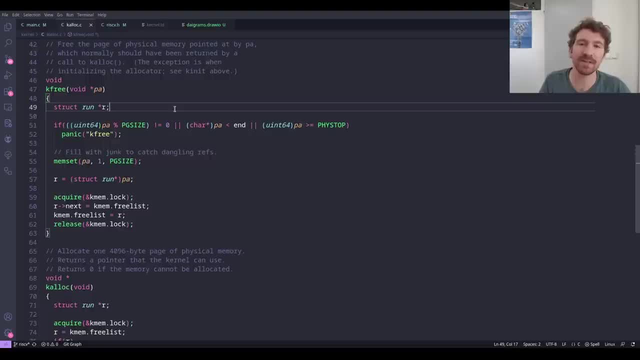 that's you do that with k alloc, allocate some memory that's similar to m alloc, right memory alloc for the k free function. So we call k free on this pointer. that brings us down to this function. This is k alloc kernel allocation And of course it mentions here that the exception is: 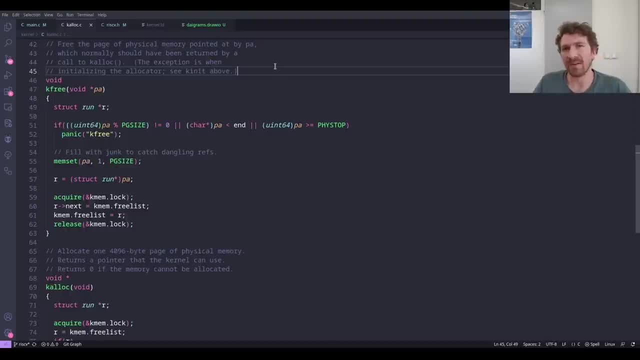 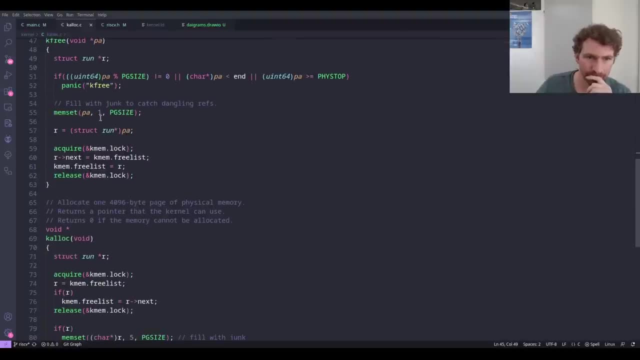 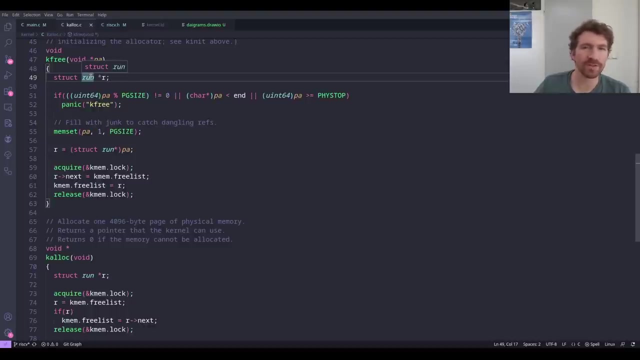 when initializing the allocator ck in it above. Well, we have seen that, so we won't go back to it, But we can use the same mechanism. Okay, so what do we do here In k free? we first set up a pointer to a structure. one of these run structures. this is this linked: 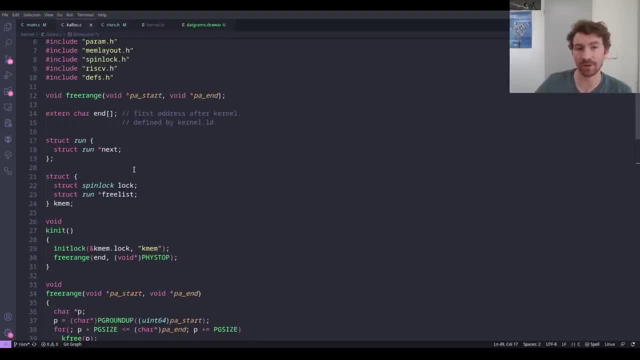 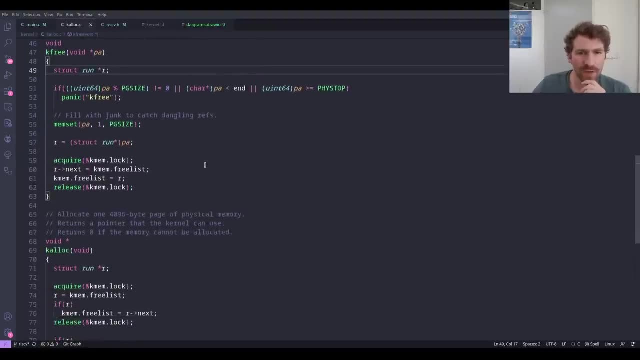 top this. that's just basically pointing to the next run structure. So we've got a kind of working pointer to a run structure that we can work with And first of all there is this kind of invariant condition. So basically, if this condition is broken, then there's something wrong and we have to just crash. 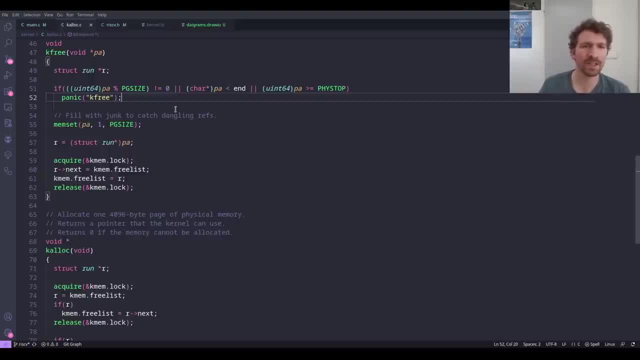 the system. it should never happen. we check it. this is something that you could remove if you wanted to, like you know, if you were really sure, but you know in essence you probably wouldn't. This is just what you would call an invariant. If this is broken, everything else is broken. 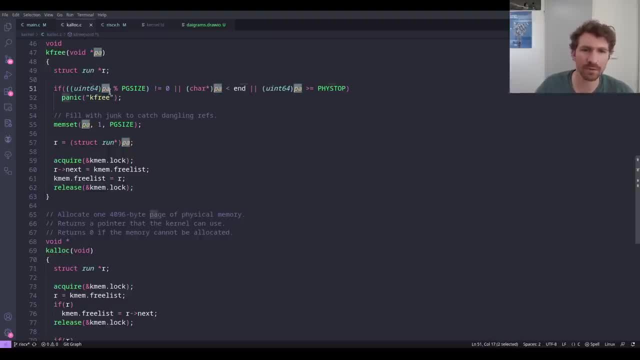 Okay. so the idea: the first thing that gets checked is: is the physical address? is it a multiple of page size? that's what this is checking, right? If it's not a multiple of page size, that means that we haven't kind of aligned this. 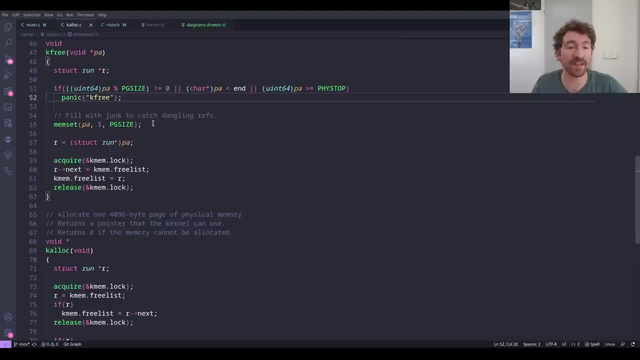 pointer to a 4k boundary, that that's not going to work for us, So we would crash in that point. So again, if our pointer, our physical address, if it happens to be like an address that happens before the end of the kernel, So if it's like part of the kernel, the code, the data, 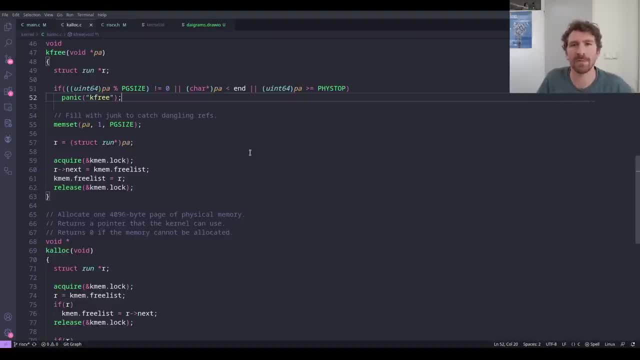 anything like that, that's also invalid. We can't free something that's part of the kernel because that's not part of our free memory. So that would also be a crashing condition. And if the physical address is bigger than the amount of memory we have, well of course we can't free that memory. 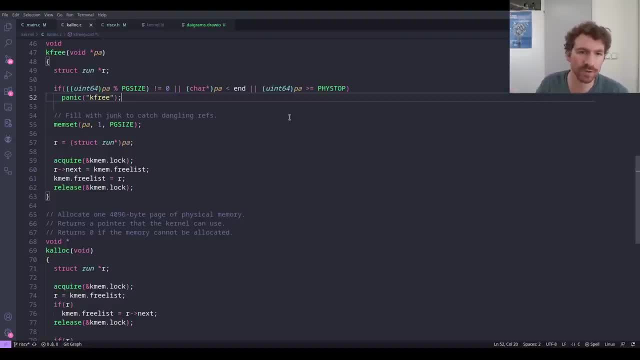 because that memory doesn't exist. So게 then we would, then we would panic and in all those conditions we just panic with K free in. in actuality, of course, that this kind of thing, this is a fun like trade-off that you see throughout the the code base here in order to you know. 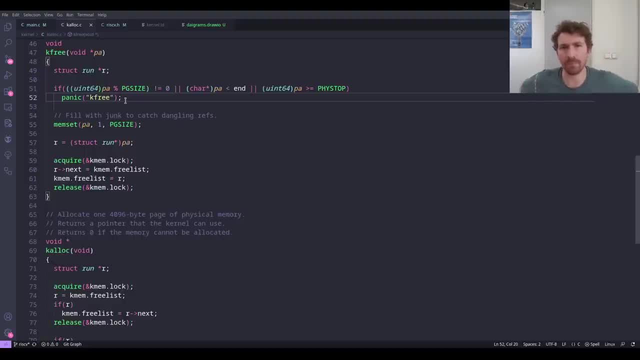 in a kernel, you have a different mindset to when you're programming applications. in the kernel, everything is about resources and just being really careful about your resources. you never want to make any code path longer than it needs to be, because any time that you're running in the kernel is time that you 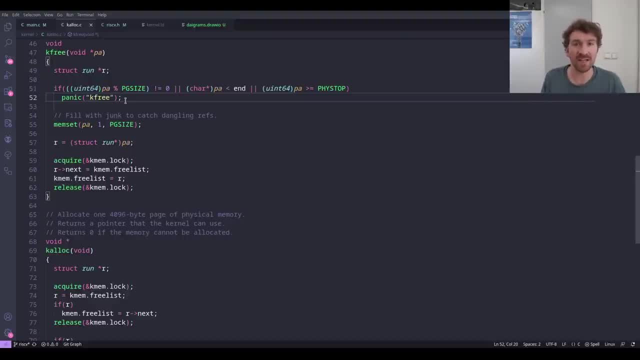 can't run people's processes in user space and, in the end, user space processes. that's the actual usefulness of a computer, right? if you're spinning away in the kernel doing stuff, you're wasting time, essentially. so what you'll see is that all three of these conditions they all just map into this. 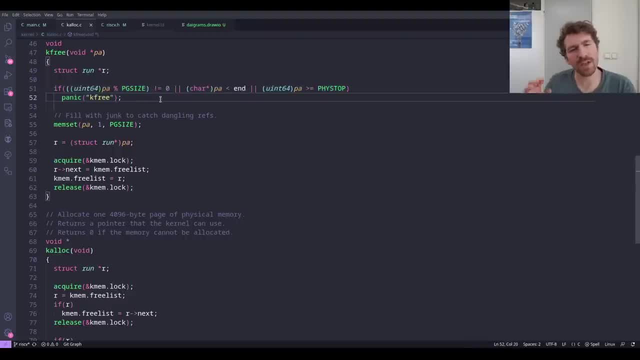 this single, this single thing, and, of course, another um thing that you don't want to do is to just like, uh, uh like, use too much memory. it's sort of the same thing in a way, but you, conceptually, you sort of don't want to spend too much time in the kernel, you don't want to give too much memory to. 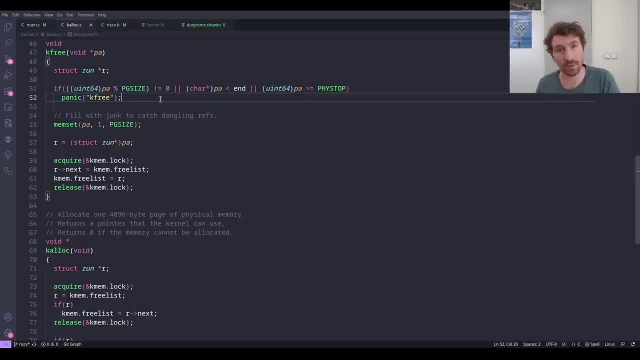 the kernel either, because memory of the kernel is memory that you can't give to processes. so, in both these cases, um, the way that this is actually constructed, is just a single if statement checking these three conditions, um, and then a single panic. you might think it would be more useful to have a panic for each of these. 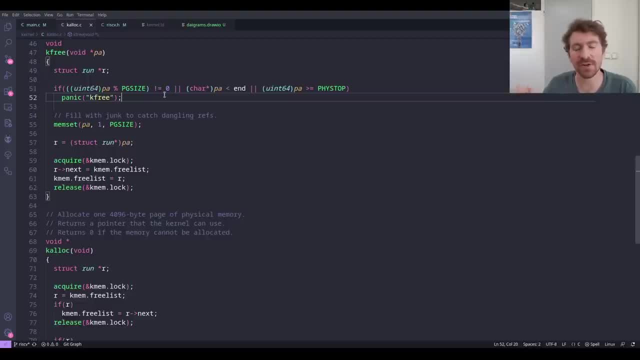 possible conditions, um, with a specific message of what happened, um. but that's kind of a different mindset. the- the kernel is- is really trying to make sure like, okay, this should never happen, and if it does happen, you know, kind of, you're probably not going to figure out what went wrong just from seeing that. 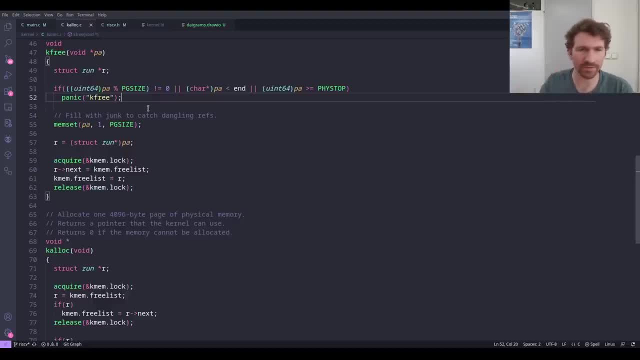 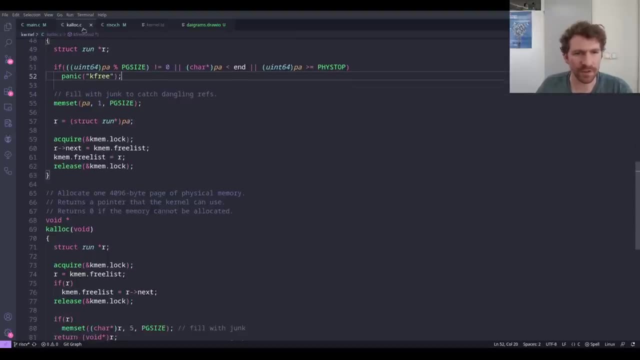 that single message. so, right or wrong, that's kind of the the mindset that's going on here with this kind of this kind of code. okay, so there's a bit of divergence, but what does the rest of this function doing? so we're trying to free this page. um, the first thing we do with the page. 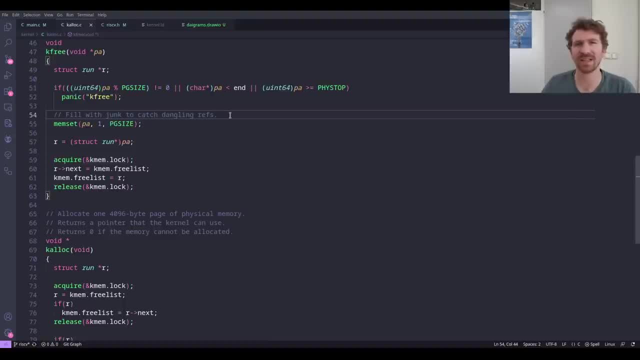 is we fill it with junk to catch dangling refs. so what's happening here is we are, um, we're using memset, set memory, so set the memory, starting at this, uh, this physical address, and for page size, so with for, for the whole 4096 bytes, set everything to one, just set every. 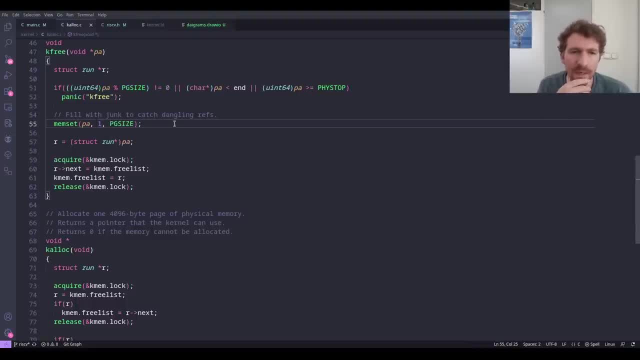 every, every byte to a one um. is it byte by byte or is it integer by integer? yeah, it looks like it's like in units of uh, u, u32, so it wouldn't actually set every byte, it would set every u in 32.. okay, but we're gonna fill um, fill it with junk. 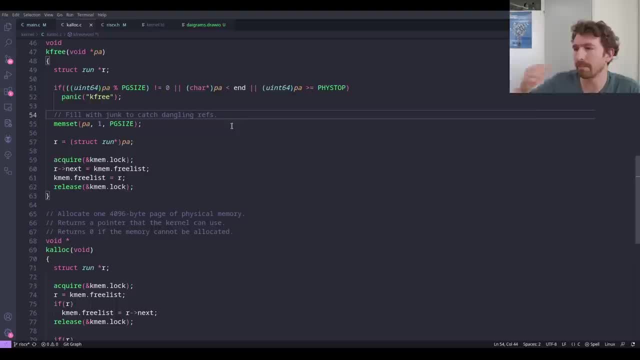 and what does this mean? this dangling refs? well, basically, um, you know, user space programs, they, um, they, they're gonna fill their uh filled memory with variables and things like that, and some of those variables are going to be pointers, so you're going to have uh things that point into memory. 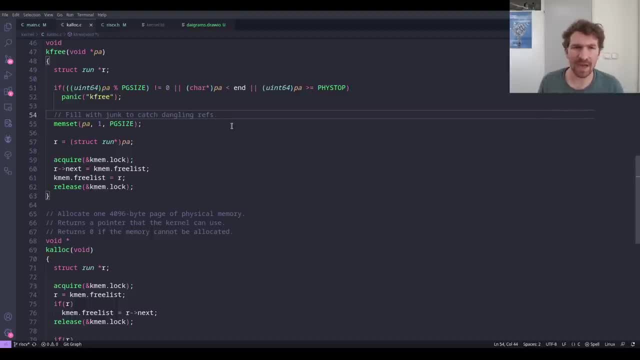 now, if you free a page of memory and somehow a user space program still has kind of like a pointer into that, but it's kind of been freed, um, well, there are. basically what's going to happen is you're going to read a value? that's, that's. 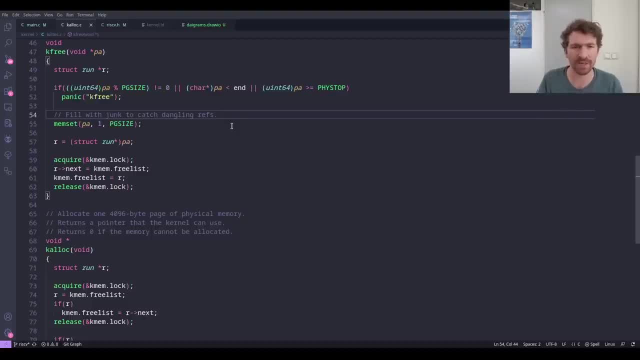 kind of stale or old. that's kind of like a use after free problem. um, if you get into a condition like that and you read back the value one instead of the thing that you were expecting to read- especially if you had like an array of items and you were just reading these ones- well, this is a way. 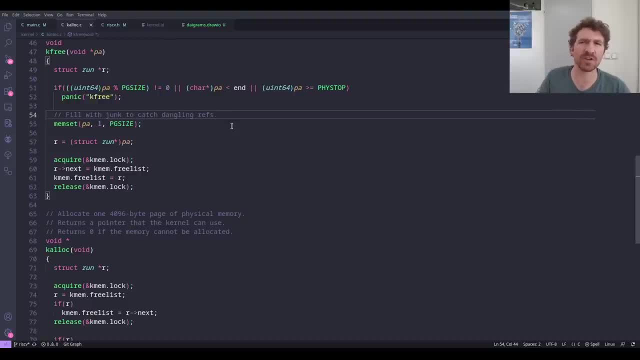 that you would be able to catch that as an issue, and this is especially relevant in the kernel itself, right, if you were trying to debug problems in the kernel, um, this would be a good way of just figuring out, like, oh, it looks like i've already freed this page. 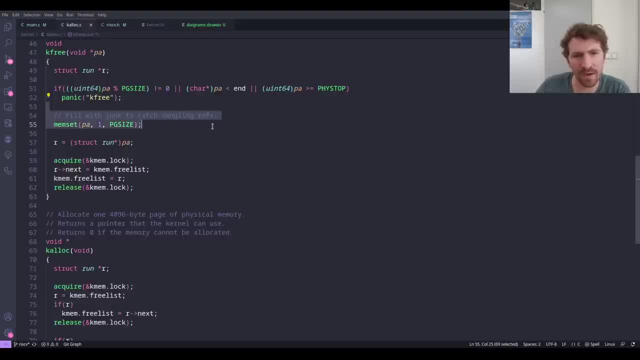 okay. so what do we do actually? so we've, we've, just we've, we've set the whole page to be one um, what we do now is we actually take that physical address which points to the beginning of a page and we cast it to a pointer, to one of these run. 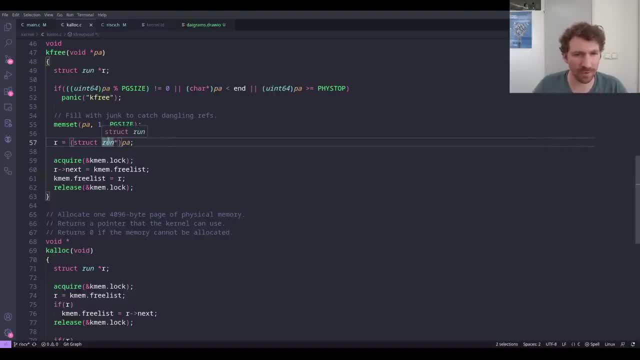 structures. so remember, this structure run, it's- uh, it's this thing here. so this is a bit of a tricky thing, and we haven't- actually, of course, we haven't- done anything with the, the memory itself. we've just got like we've got a pointer to something here and we're 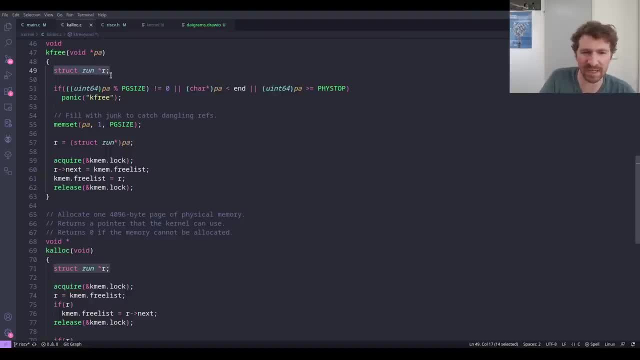 saying like, okay, the thing that this points at the area of memory is over here. so we're just like basically telling our c compiler: uh, no, this random address, oh, it's definitely, it's definitely a run structure. no, it's, it's a run structure. i've checked it and i know for sure it's. 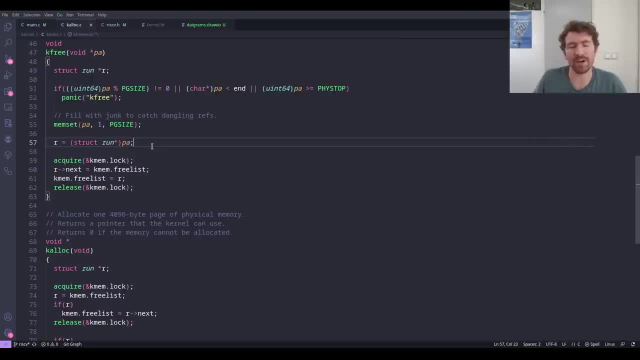 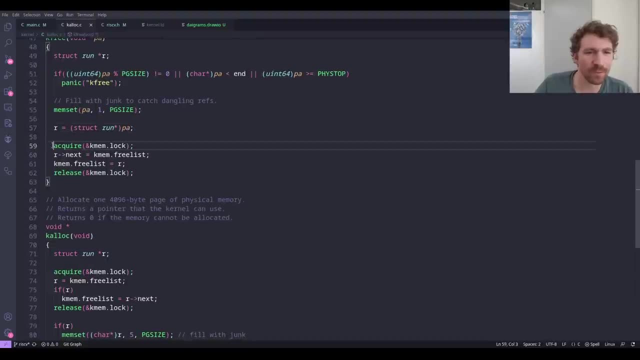 a run structure. of course it's not right, it's just random memory, but we're sort of imposing the lens of it being a run structure now. and so what do we do? we acquire the lock and then we release it afterwards, so we're just making sure. 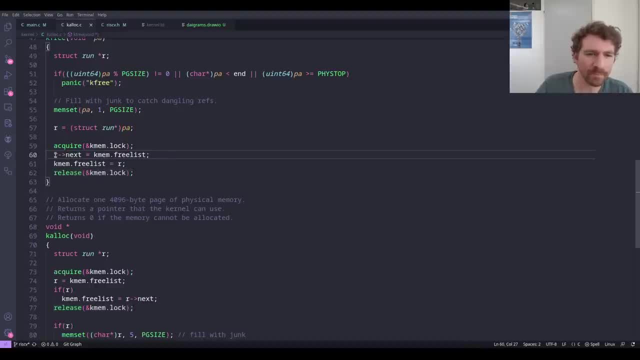 we don't collide with any other cpus here and we we set the r next. so basically we're going into the memory, the physical memory of this, uh, of this system. now we're going and writing, uh, the very first um, like 32 bytes, uh, sorry, the 32 bits of. 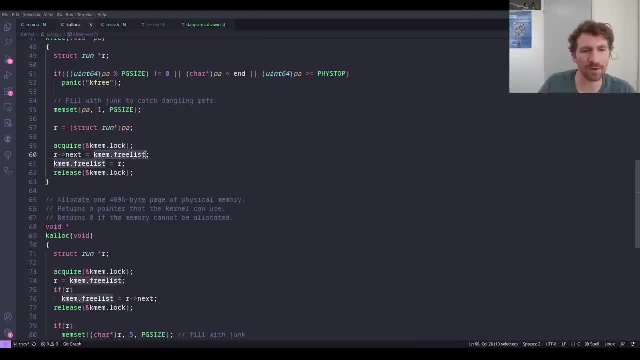 it. we're writing it to be the address of. sorry, i guess this would be eight, eight bytes. since it's a pointer uh in a 64-bit system, we're writing the first eight bytes to whatever our currently uh pointing free list is. so remember we've got this km and we've again got a. 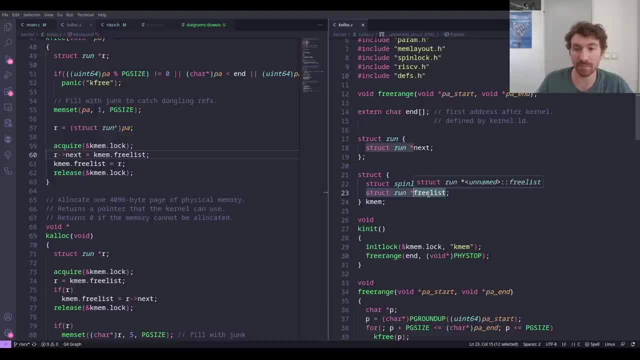 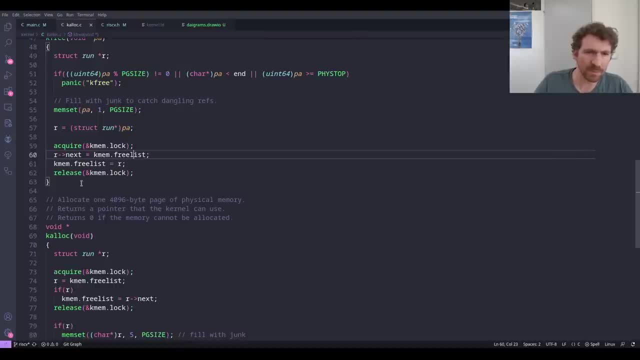 pointer to a run struct here. so in the beginning, when we first boot the system up, this is going to be pointing to null. it's going to be a null pointer. so what we do is we set the pointer of of this thing to be, uh, whatever the last one was. then we say that our new free list. 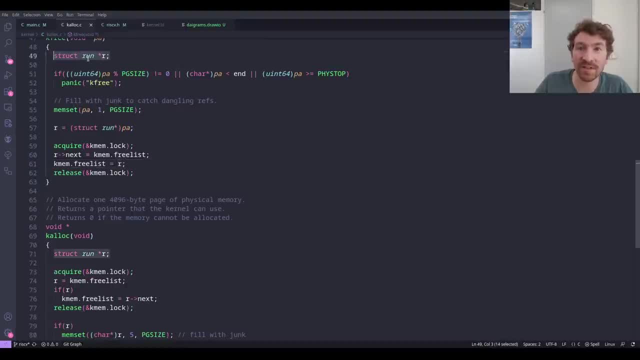 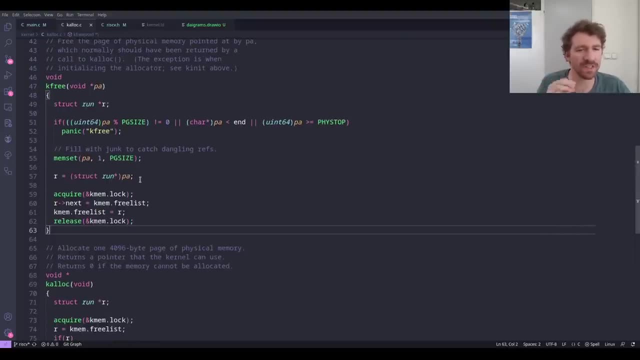 is this random run structure, this pointer to a run structure, and then we release: now you? this probably doesn't make a whole lot of sense to you. this is a kind of piece of code that i think is really tricky to understand, even if you're, like, familiar with c. 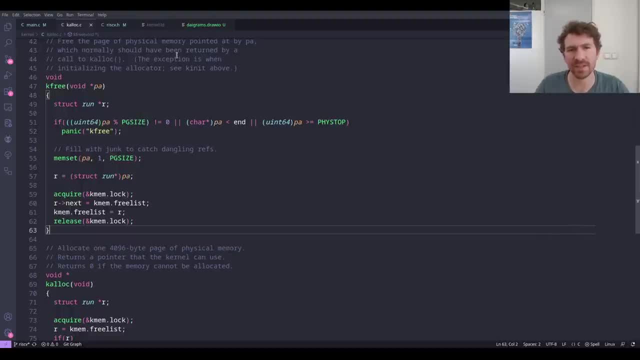 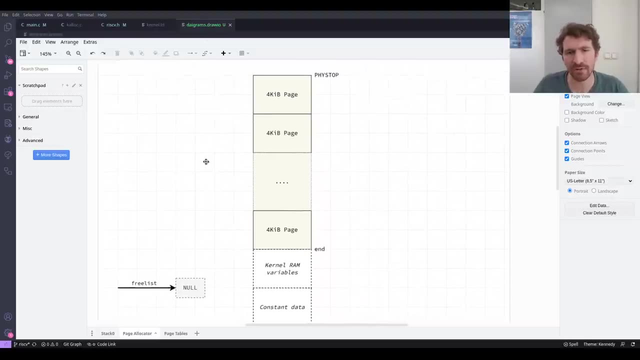 i think that reading this kind of code can be tricky, so let's actually look at a diagram to make this easier. so what i've, what i've done here, is i've kind of diagrammed out the memory of the system. so down here is the kind of the very 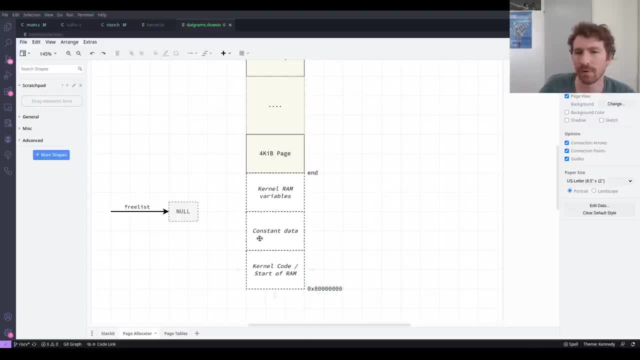 bottom of memory. this is where the kernel code goes. then we've got our kind of constant data, we've got our kernel ram and our variables and then kind of, after all of that stuff, that's where our end begins, right, that's, that's the end of all the kernel stuff. 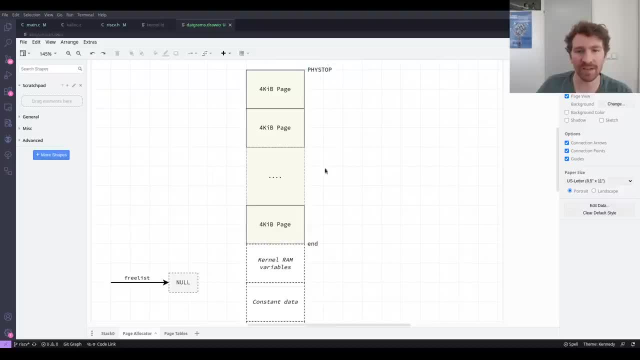 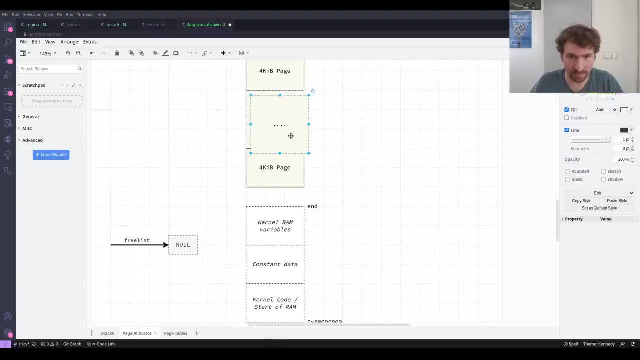 and then everything after that until the end of memory is just made up of these 4k uh pages, and i guess one thing that i should have drawn in this uh in fact, is that this could be kind of not aligned properly, so maybe i should. i've put something in here just to show that this sort of isn't aligned. 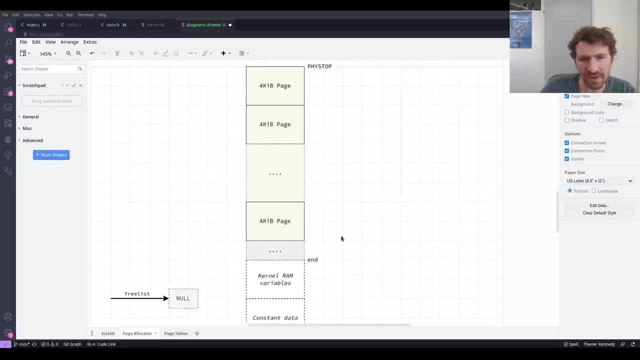 necessarily all right. so everything from this point onwards is, uh, four kilobyte pages. there's tons of them. there's going to be a lot of them in the system at that point. and what are we doing? so this? let's just imagine that we just tried to free this. 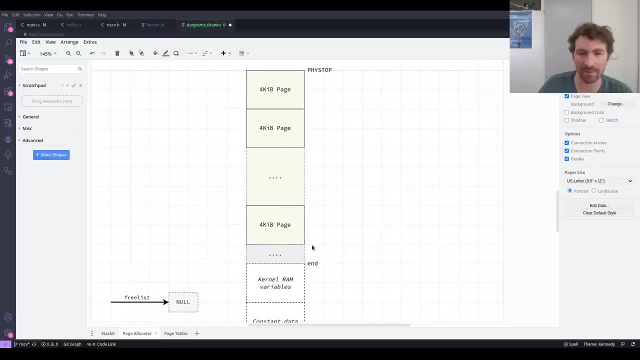 very first page of memory right. so we got our address, we rounded it up to the nearest four kilobyte boundary and now we're going to try and free this page. so what happens? well, first we check all of our conditions right. we check that we we're not like we're properly aligned, that we're not. 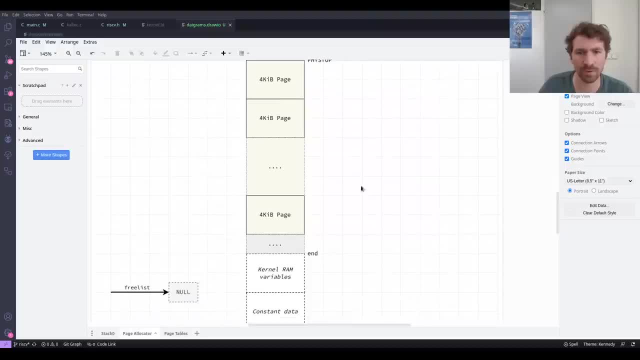 uh, like down here that we're not beyond the physical top. uh, so okay, all of those are good. then we're going to set every um, every uh value inside this to to one so that we can kind of debug if something goes wrong. then we acquire our lock, so we block any. 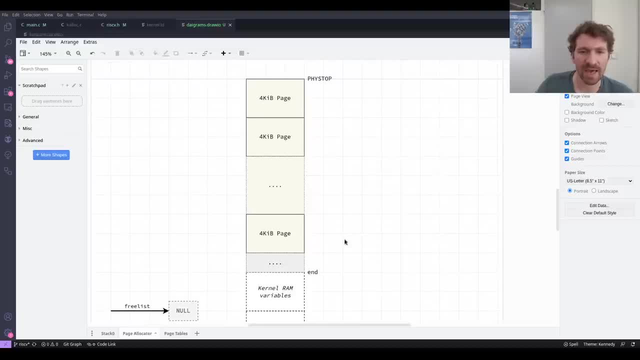 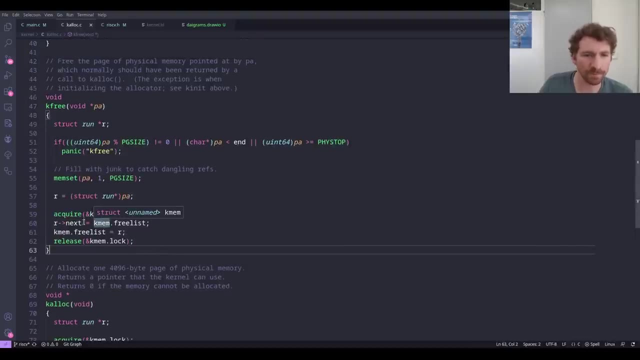 other cpus from doing anything with the memory at the same time. and we, uh, we set the the next of our free list. sorry, let's make sure we do this in the right order. so we set the pointer, this new pointer that we've got. we set it to be equal to our- uh, our old free list. 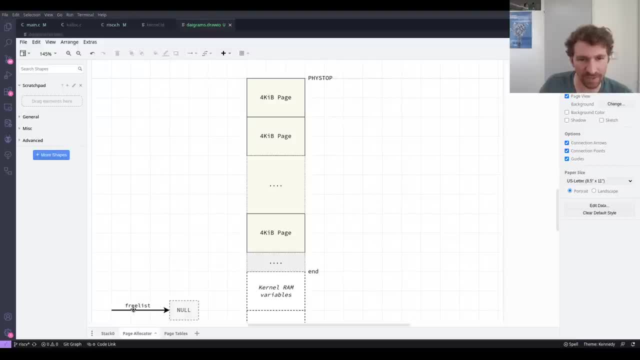 okay, so what's that going to look like? well, this is our kind of our free list, um, so our old free list is pointing here, so that's going to maybe look something like this: we end up, uh, kind of writing down that we're pointing down here, and then 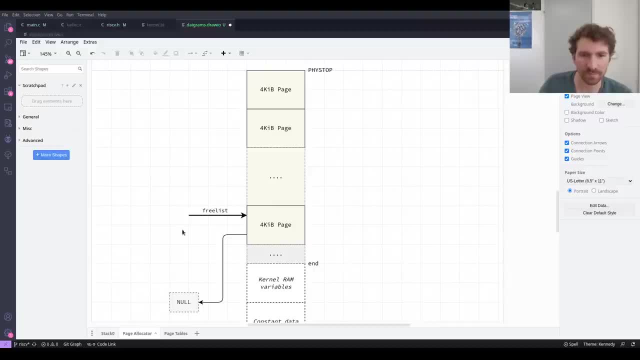 we set our free list to this page, so that's what's happened here. so now, um, if we kind of zoom in on this- and i'm going to try and make something on the fly here, which is maybe not the best idea- if we kind of think about, like just uh, like this page as being, you know, a 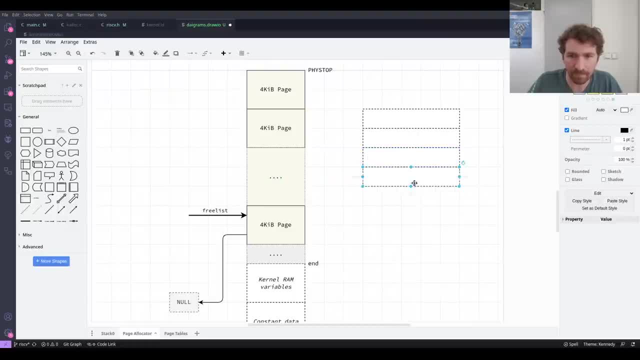 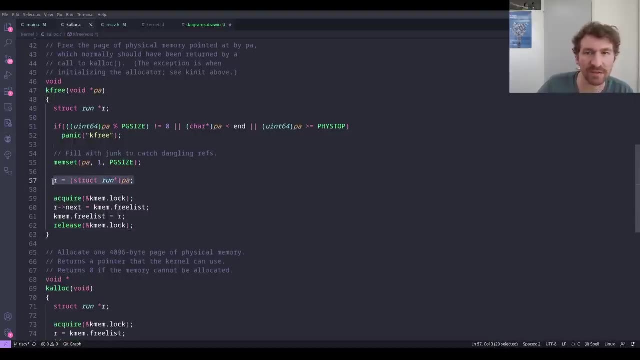 series of um things in memory. well, in the beginning we've like these are 32, uh, 32 bits at a time, so we've kind of set everything to one in the beginning. but then what we're actually doing at some point is we are, um, we're saying that, like the beginning of this, the first like from 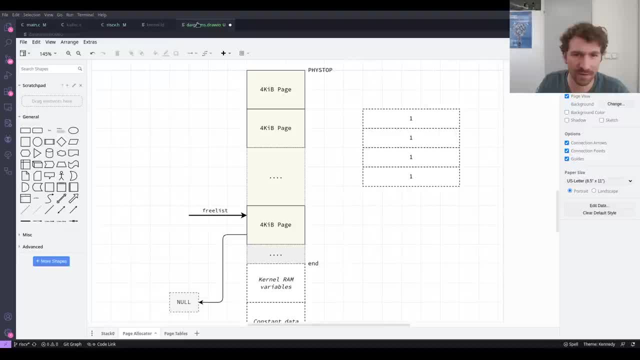 like. we're casting this memory address that points to this page. we're casting it to a run structure, so the run structure has a next. so the very first thing in here is now the next, and we're pointing it at our old free list, so this now becomes a. 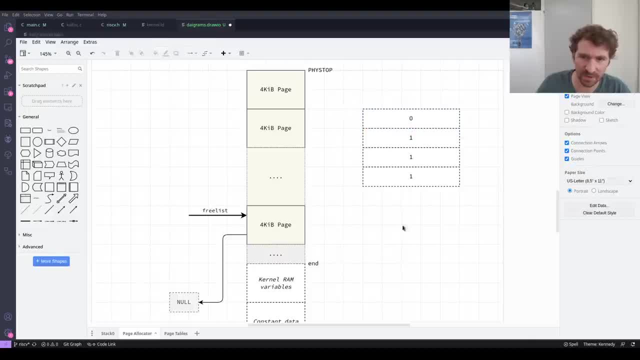 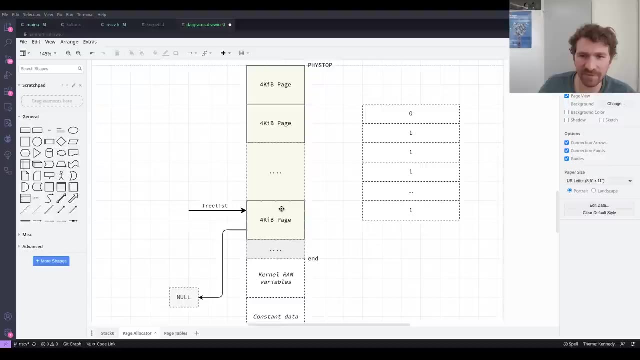 a null pointer, right, this is. this is kind of like, uh, this is kind of like a representation of what any of these 4k pages looks like. okay, so what we've done is we've, we've pointed down here: uh to null. that's the old free list, and 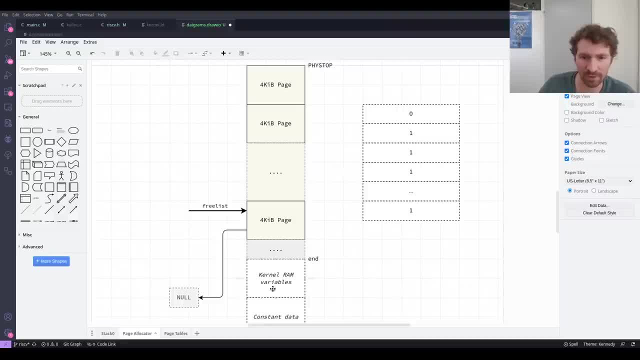 we're saying our, our free list, and this is going to be a pointer that lives somewhere in here, right in this, this part of the code, our free list just points at this. the new page, that's the next free page, so we freed one page. if we were then going to allocate a page, 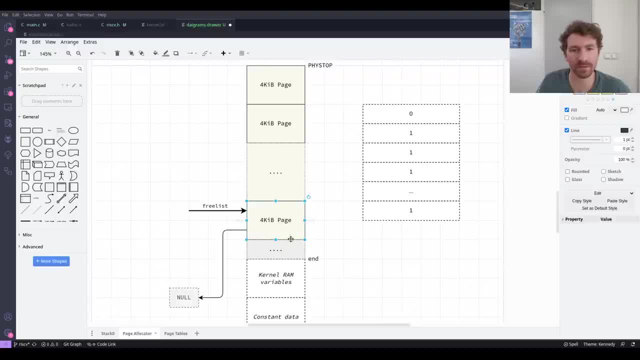 we've actually got one to give. now we can give this page, so that's how this is going to work. let's imagine we freed another page, right, so we've got the next page along. let's- uh, let's- grab- move that up there a little bit, so we've got like a new page to play with. 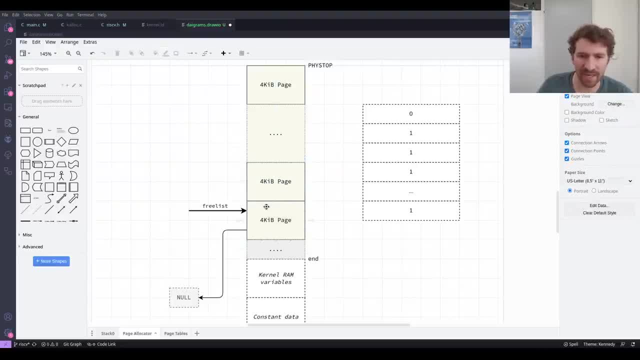 so this is the next page. right, we started down here. we're going to add 4k, so we're now going to be here. i'm going to free this page. so what do we do? we set everything to one again, of course. so this is our new page. 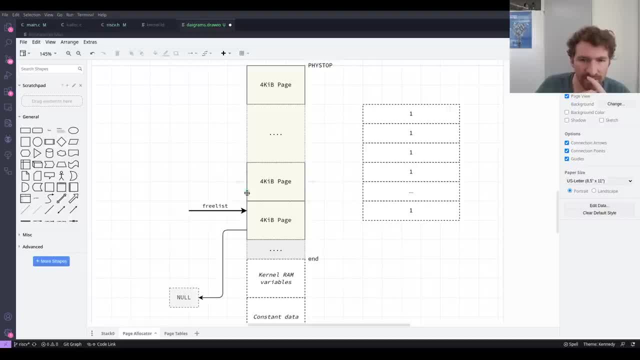 set everything to one. then we take the pointer here and we're going to kind of point it at the previous free list. so what's that? that's going to be basically pointing to this area of memory. so we're we're kind of pointing down to the previous page. 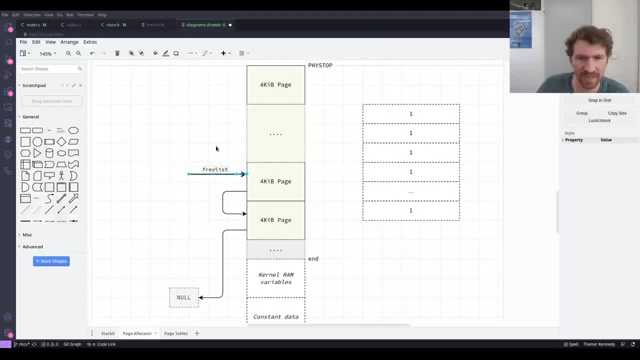 and then we take our free list and we point it here at this page, and of course, what that means is that this one is kind of going to be like: the address of this is going to be page roundup end. right, that's the address that's in in the free list. now, right, we're pointing. 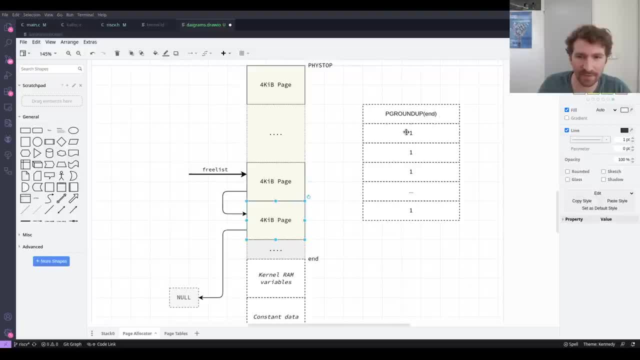 sorry, that's the address that we put in our, in our next like, whatever the like, the next page that we could give. so this is the first page we can give. this is the next page that we can give if this one gets freed. and then, of course, we're just. 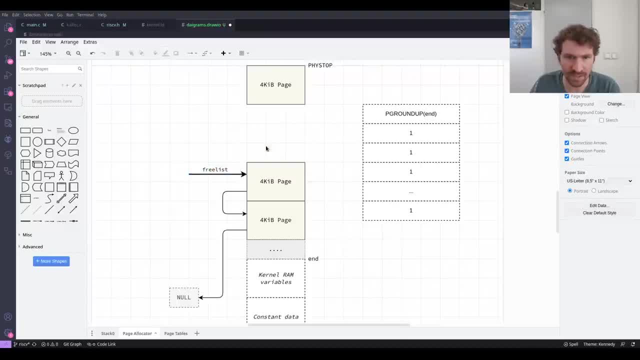 going to continue this process. so, um, let's, uh, let's, get rid of that, let's actually put in just like a couple more pages and then we can see the final structure on the fly drawing here. so we're just going to end up essentially um disconnect that take this. so we end up in a structure that looks kind of like this: 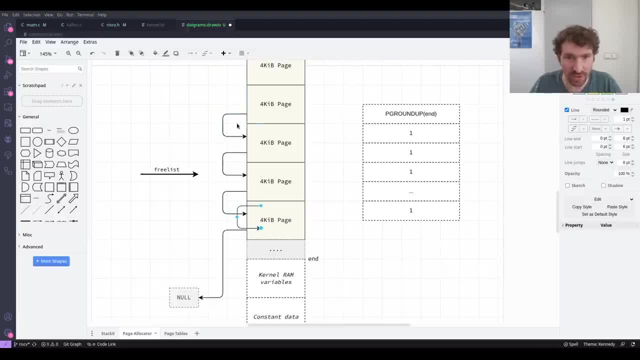 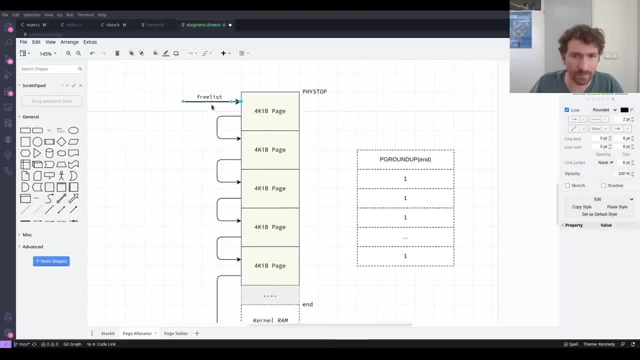 with um each page, kind of pointing back at the, the next one and then something like this: so the free list is going to start at the very, very end of memory and that's kind of an interesting thing like: uh, it's a if it's a fun way of building a linked list. i think people like you naturally imagine that when you're. 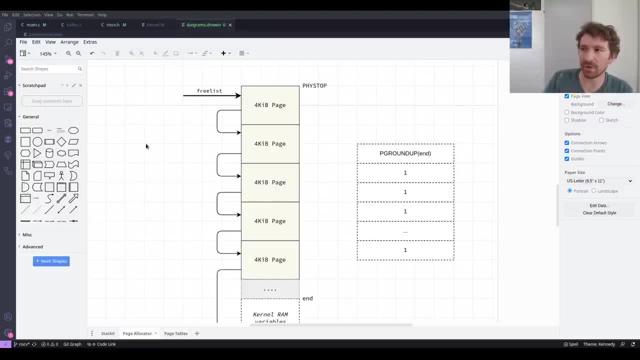 building a linked list that kind of. you start in the beginning and you point to the next thing and the next thing and the next thing. and the way that this actually builds it is that it kind of shifts things in from the bottom, so, but by the end you're actually pointing to the 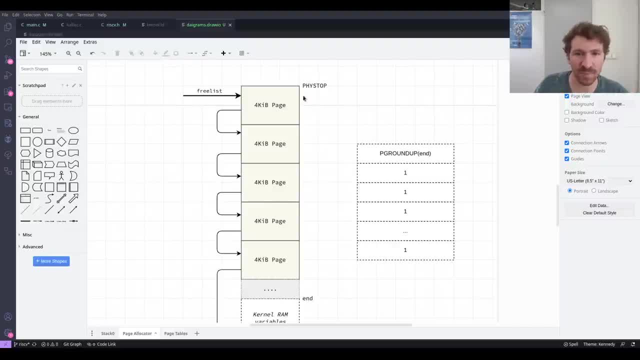 the last item in the list, sort of conceptually speaking, it's the last item you dealt with, is the last i the first item you you point to. so we end up like, if we're going to allocate a page of memory now, we're allocating from like sort of the very end of ram, so that's where we would allocate. 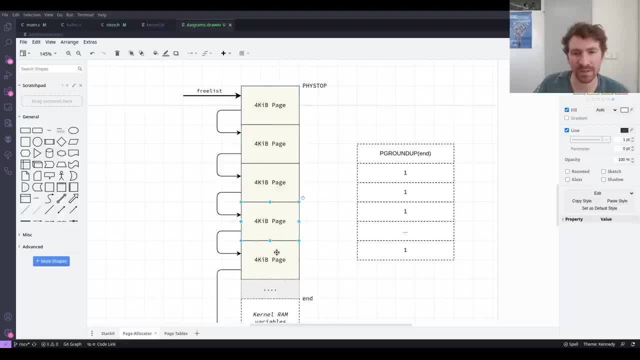 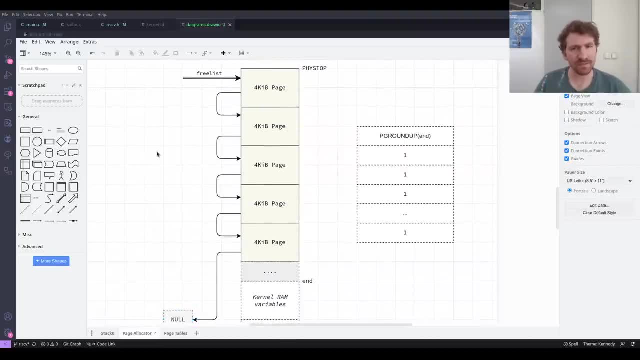 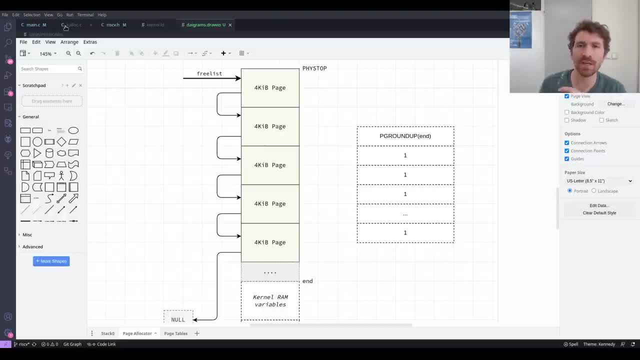 really surprised me about this diagram is that it's a bit tricky, um, i think. and what really surprised me about this when i when i read through the code, is that i imagined that in a kernel you would have sort of some structure somewhere that would somehow keep track of all of the free. 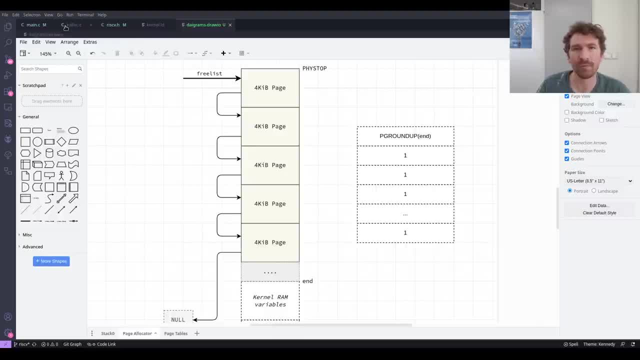 pages, um, so you would actually have just a piece of memory that was kind of a table and it said, yeah, okay, this page is free, this page is not free. maybe you would have two tables, but in fact that's kind of not what happens. the the memory itself is the data structure. that's kind of like, i think. 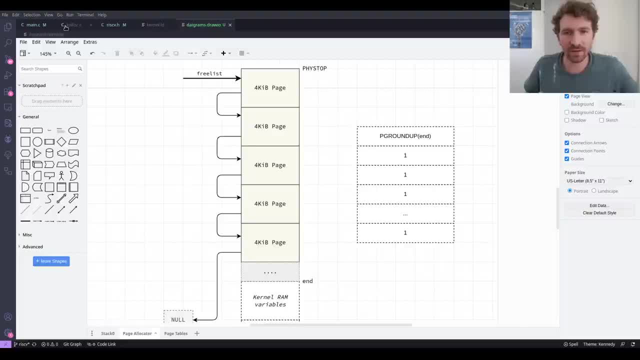 it's kind of like what's it like? a bit like a little bit more like, uh, a bit more like a bit more done now. right now. it's kind of kind of a mind blown moment. it was for me like that- that we actually use that memory itself as the data structure that keeps track of which pages are free. 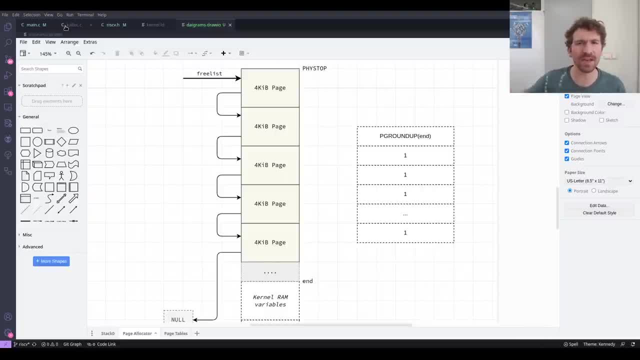 this kind of the beauty of c and having things like pointers is that you can do this. you can just say that random memory address over there: yeah, that's a linked list node. uh, actually it's sort of like a kit, a four kilobyte page, but actually it's just a random memory address we can. 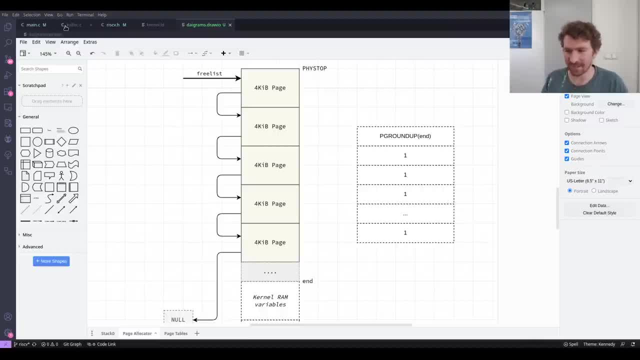 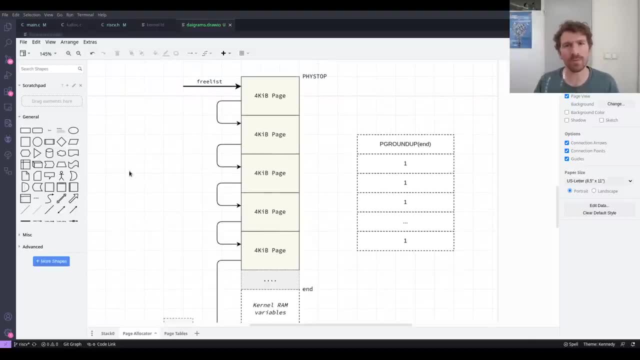 Its first element says where the next next thing is. And if we kind of follow those through now, all of a sudden you have tracked all of your physical memory that you have to, to, to, to give away And you haven't had to use any memory to store that. It's kind of mind blowing because all that memory is free, Right. 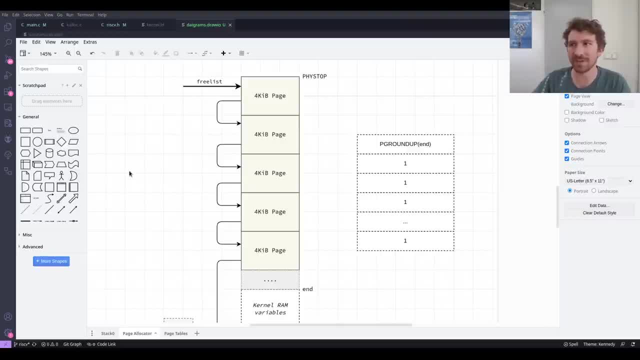 It's not being used for anything And the minute that you want to use it for something useful, you no longer have to use it to keep track of what's free, because you only ever keep track of what's free. You don't keep track of what's being allocated. I hope this makes some sense. It is a tricky concept. 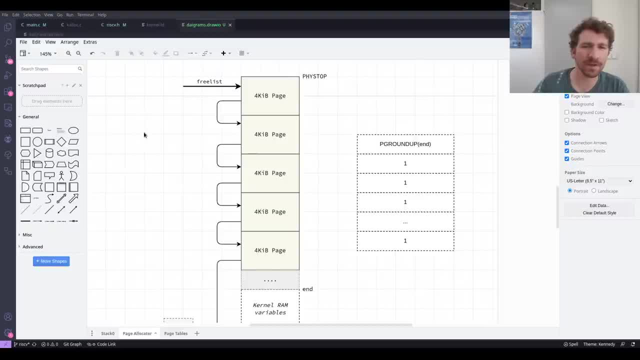 So if it's, if it doesn't completely click, Then maybe try and download the code and step through it in the debugger, kind of try to write down physically what's going on. like what would the address be at this point? OK, round it up, Do kind of go through these steps and see how it's working out. It's really eye opening. 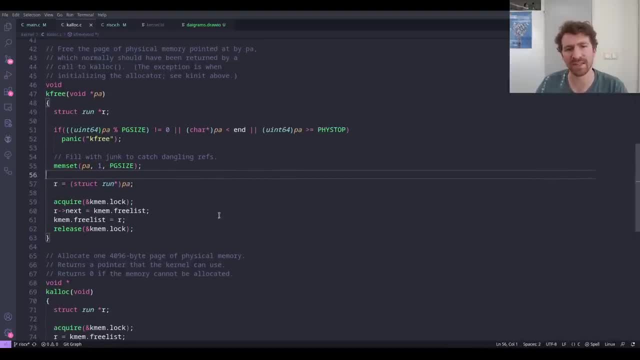 I think it's a really, really Very clever mechanism, and it's not the only mechanism, right, This is certainly not the mechanism that's used in Linux or anything like that There are. there are different algorithms that you can use for the same thing, of kind of allocating memory within the kernel. 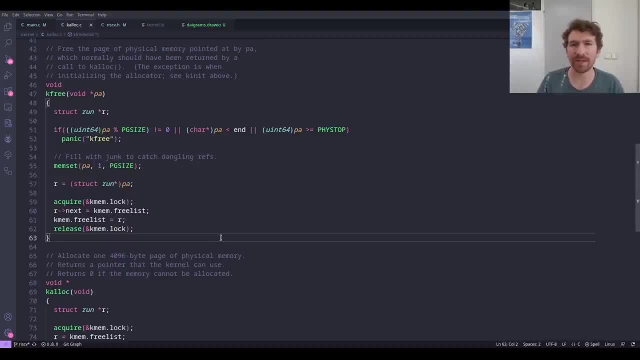 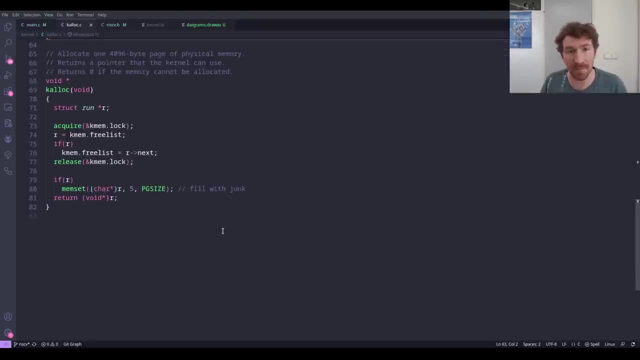 But this is a very elegant way of doing it. I think it's very beautiful. So how does allocation look? We might as well talk about the full picture here. So how does memory allocation itself work? So here in K Alex, We allocate one four kilobyte page of physical memory. 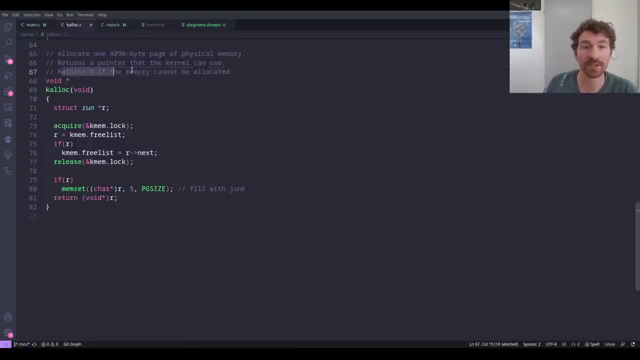 It returns a pointer that the kernel can use. It returns zero if memory cannot be allocated. So why could memory not be allocated? Well, because there wasn't any right. That's. that's, that would be the thing. So, basically, we're returning a null pointer. in that case, 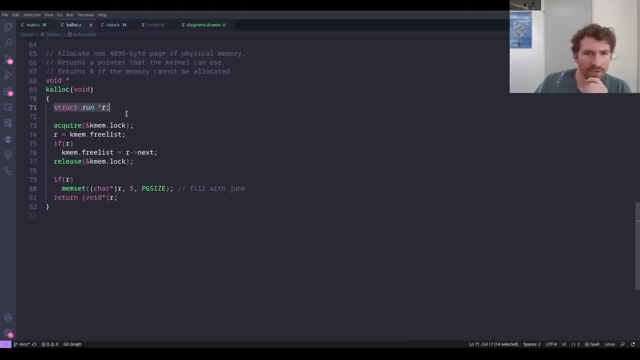 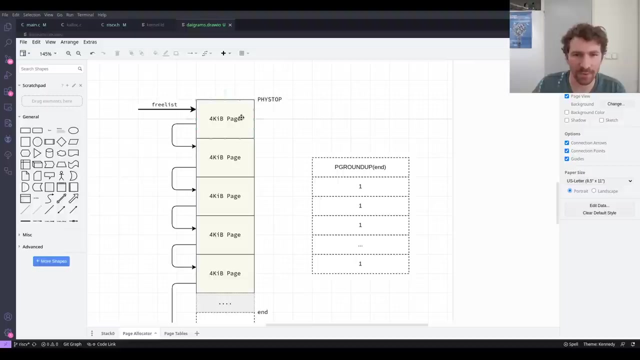 All right. So what do we do? We keep track of the local run structure. We acquire the lock. Um, we basically say that, uh, that's equal to whatever the free list is at the moment. Keep in mind again that our free list is just pointing out whatever are currently most free pages. 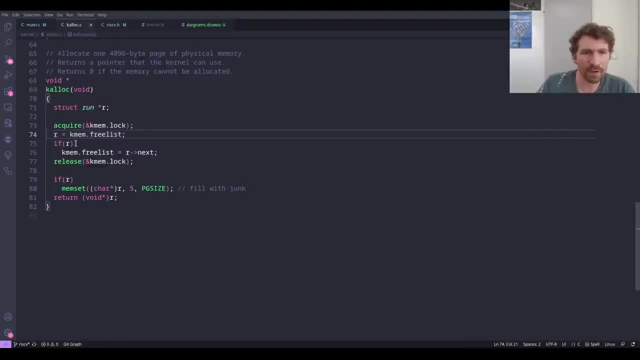 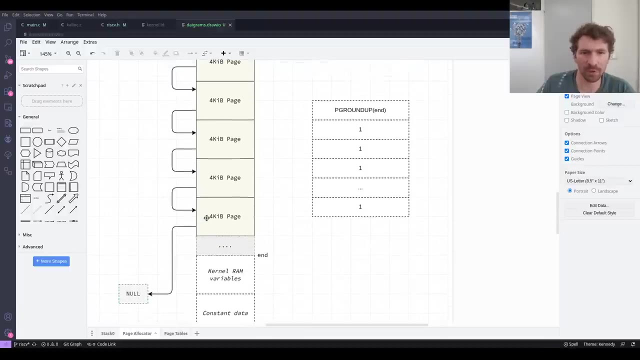 Uh, so basically, if we, if we got something that wasn't zero, I um our free list wasn't down here pointing at null, It was pointing at, like one of these valid pages in between. If we have that situation, then great. 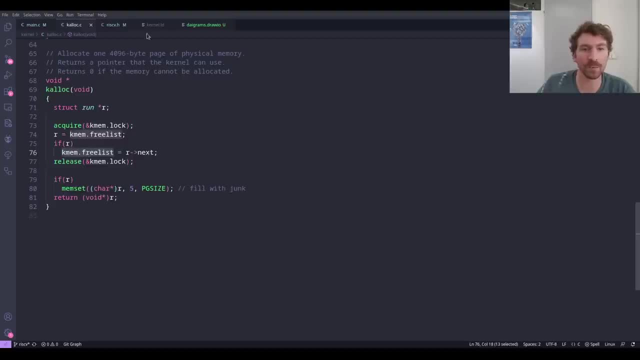 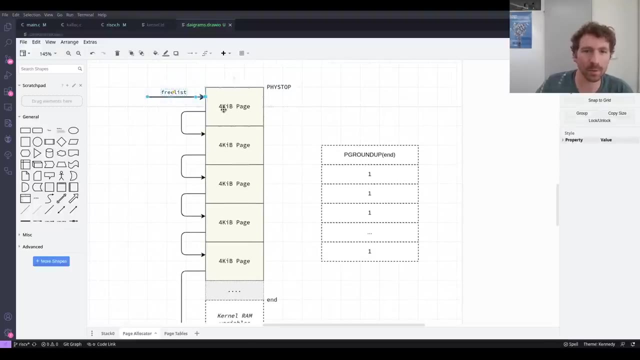 Uh, what we can say is that our free list is whatever the next one is, So let's have a look at that. What we're basically doing is we're sort of keeping track of what this one is. That's the one we're going to give away. 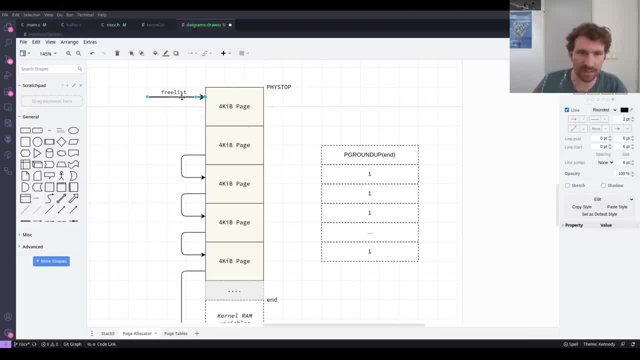 And then we say, okay, the free list, Uh, now the free list is pointing at this one. So we've got this page. It's kind of ours to give away now And that's what we would give away And we don't have to keep track of it, right? 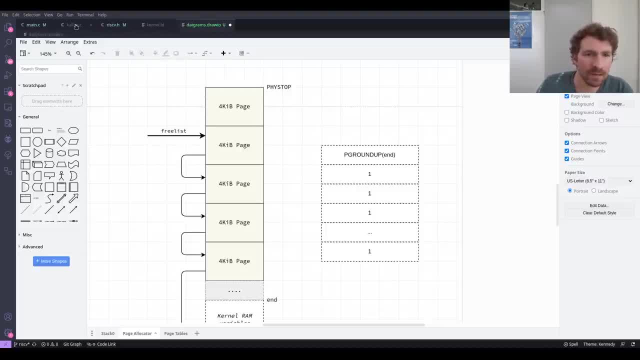 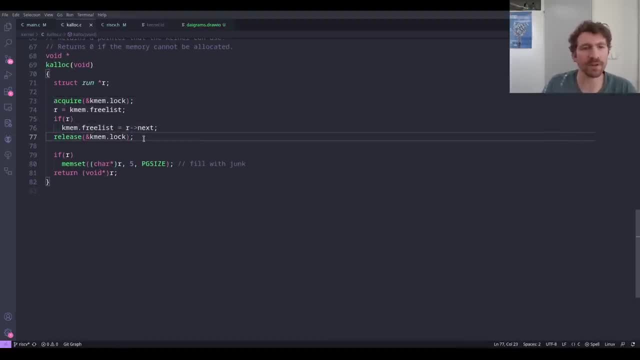 It's just like a page that's free, So that is how that works, Um, and then we released the lock. So it's a very simple Mechanism, right, Just give the first thing you have available And basically, if you, we do one more, check down here. 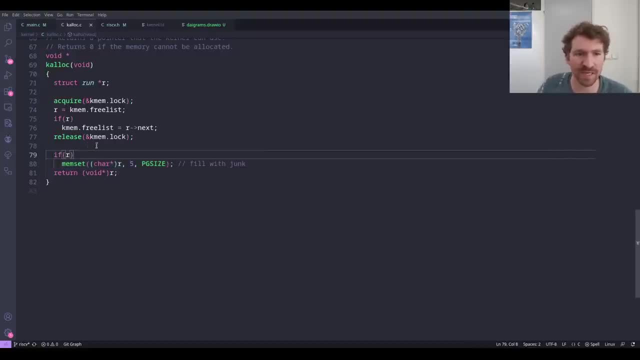 like if we got something, like if there is a page to be to be looked at, well, now we're going to set all of the uh, all of that data that was in there. I remember everything is kind of like we said it all to one before when we freed it. 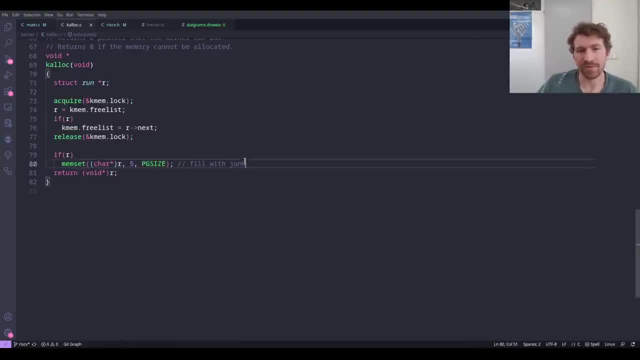 Now we're setting it to a new value, We're setting it to five, So we're filling it with junk, but we're filling it with a different kind of junk. So if it was a free page and that's kind of- uh, also a debugging thing. 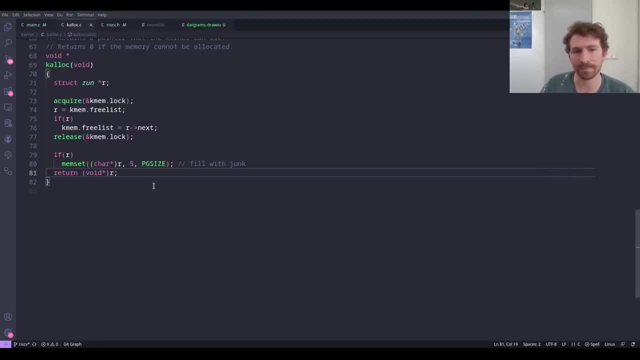 right. It's very quick and easy to see, when you're examining memory, if something is filled with a one or if it's filled with a five, And in the end we just return: uh what, we got that struct run pointer. We just convert it back to a void pointer and return that. 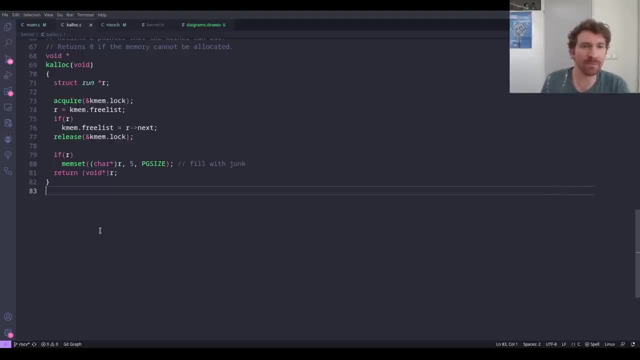 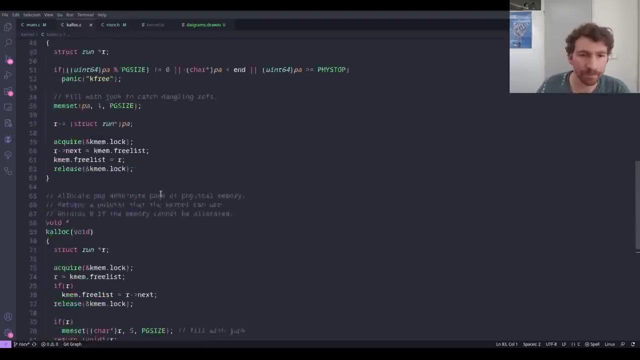 So that's it. There was no special case to check if we didn't get memory, because the free memory just points at, uh, a null pointer in the end. This is the entire memory allocation process. Um, really clever, If you ask me. really. 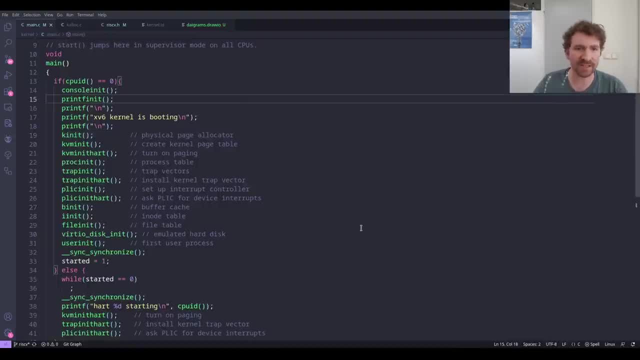 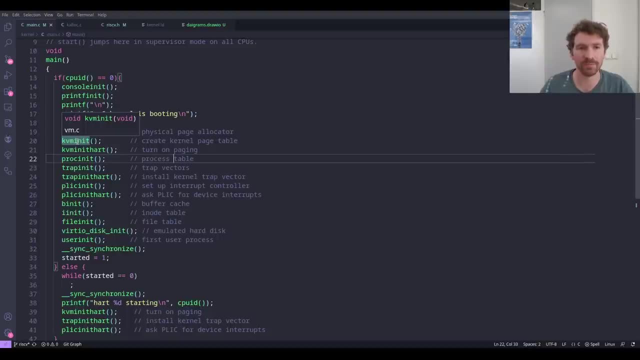 really clever And um, what we'll see is that if we uh, if we just take one peek into kind of the next function down. so we looked at K in it. we've now looked at the entire uh allocation process. 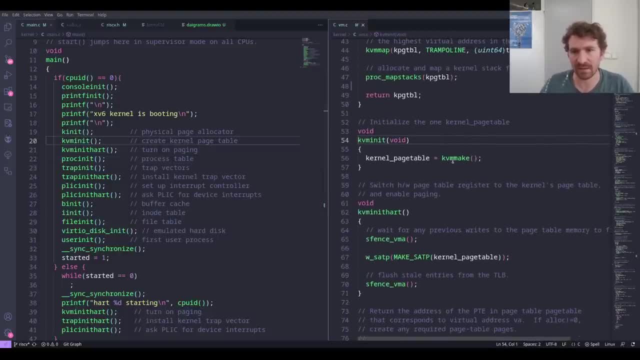 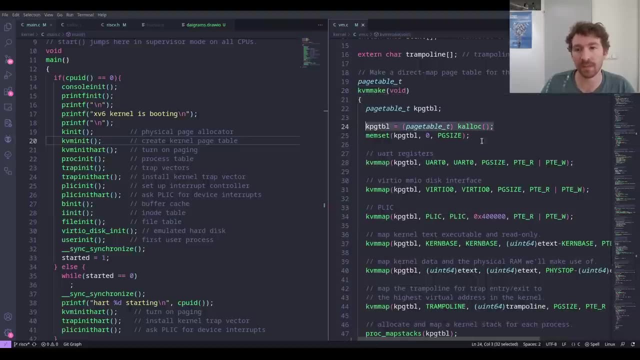 If we look at the next thing here, when we're in it and we follow a couple of these functions through um, you'll see that one of the first things we do inside this function is that we allocate a page so that we can start using a dynamic memory. 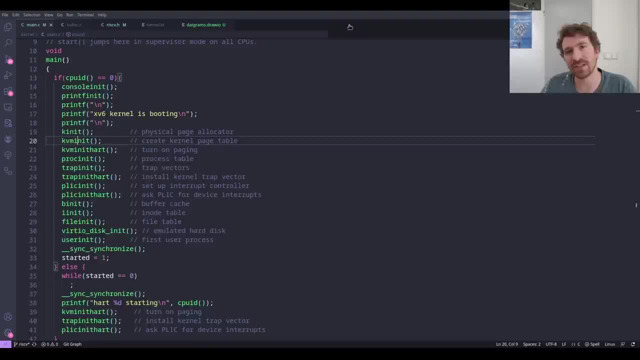 Right, Uh, so that that's. it immediately starts being used. We're gonna look into that in the next episode. Um, yeah, for me this has been a really a really fun one. Um, I think it's a really beautiful mechanism. 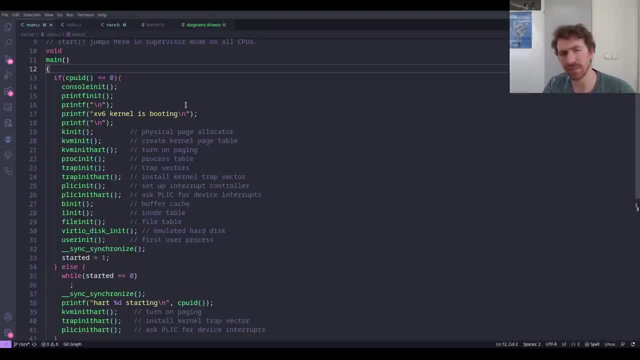 As I've already mentioned, I'm really curious as to what you think of it Like. um. let me know in the comments. Um, I'm really curious as to what you think of it Like. um. let me know in the comments. 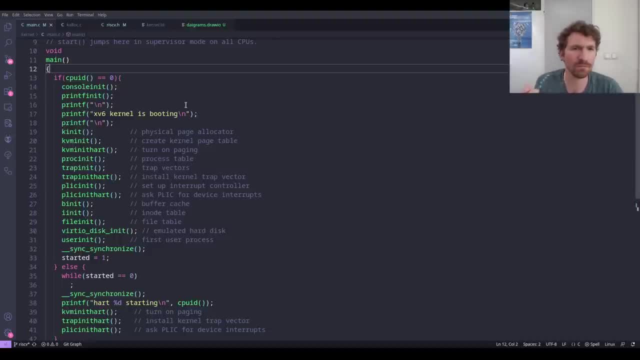 If this made sense and if you kind of have any questions about it and like if you would do it differently or if you have any other ideas, I'm really curious to see what would you make of it. Um it's. I've really been enjoying all the comments that have been coming in from people who have all different kinds of backgrounds. 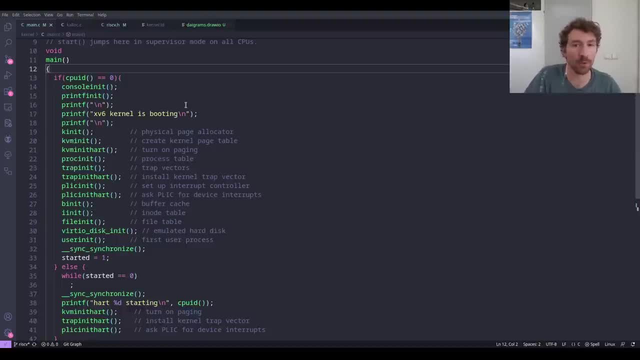 People who are doing web development but are finding this interesting. People who worked on Unix, you know, in the seventies and eighties, and are kind of being able to come and look at, look back at this. It's great. So please keep letting me know what you think of it. 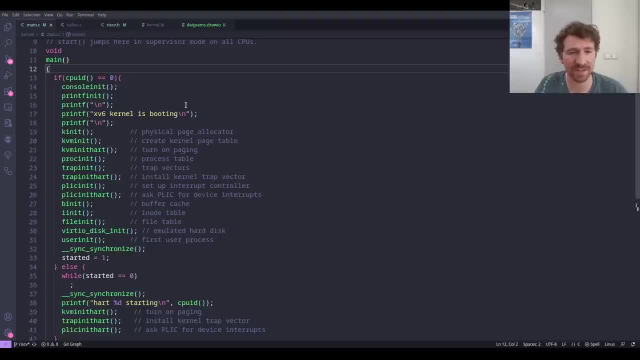 Um, if you have any interesting observations or anything like that, or questions, I really welcome them. Um, I really hope that you'll join me in the next installment of this, uh, this series, where, in all likelihood, we'll look at the virtual memory system.